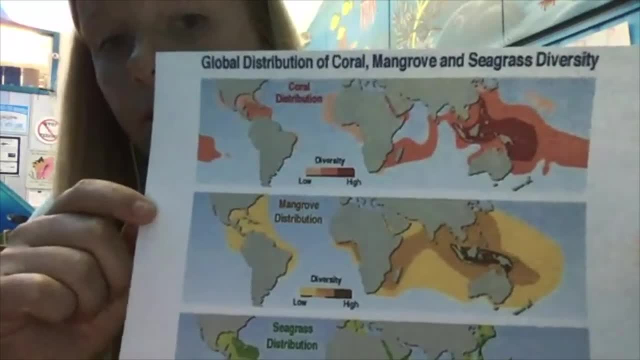 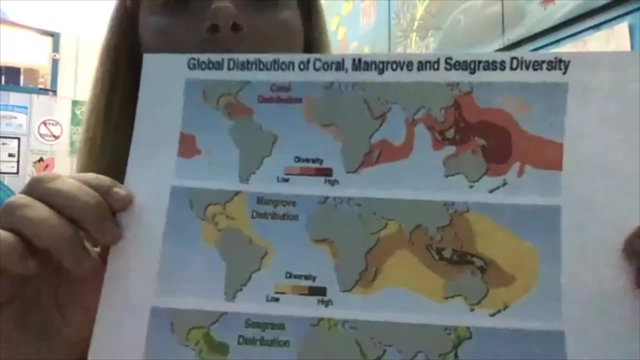 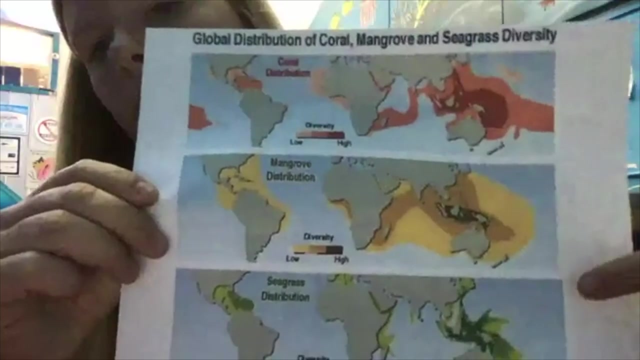 that the colors aren't 100% identical of where they are, but we can find seagrass- oh sorry, mangroves and corals in very, very similar areas If you guys take a look at, even like Australia, let's say so, right. 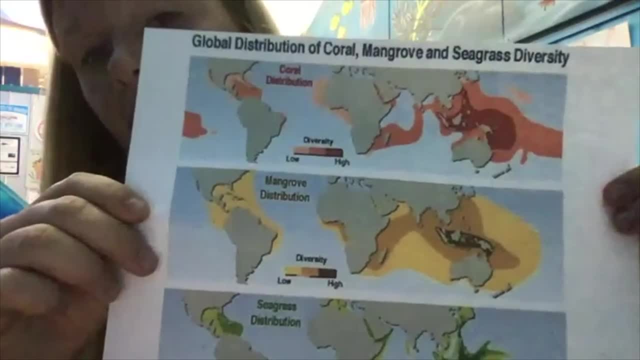 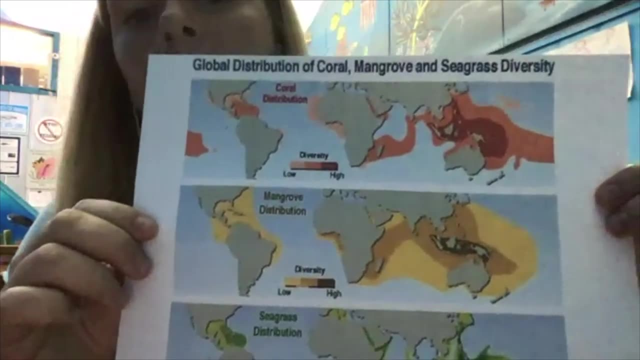 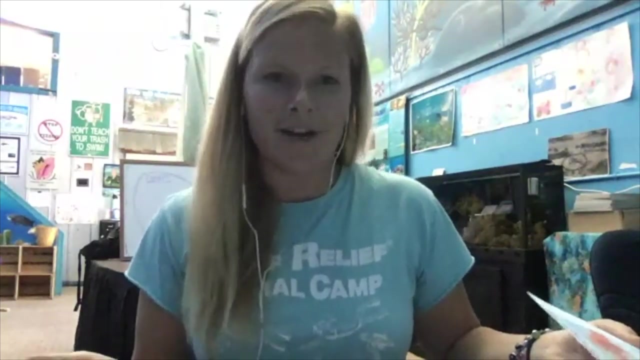 here on the map, these two guys on this side. you guys can see Australia is covered with red and Australia is also covered with yellow and that is because mangroves and corals and seagrass are all found in very similar areas. These three ecosystems need each other to survive in order to stay happy, survive in order to stay healthy, and survive as a survivor in order to value a beer or a drink, and healthy. So if we see coral reefs, there's probably going to be some. 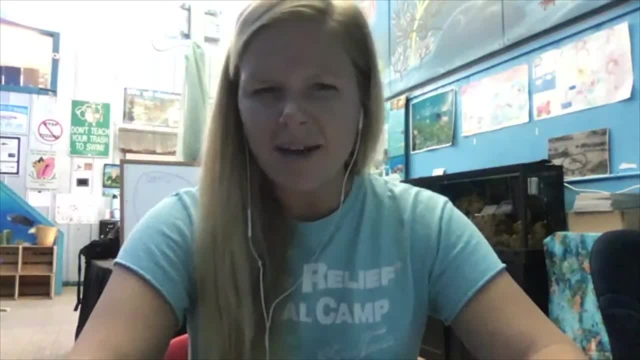 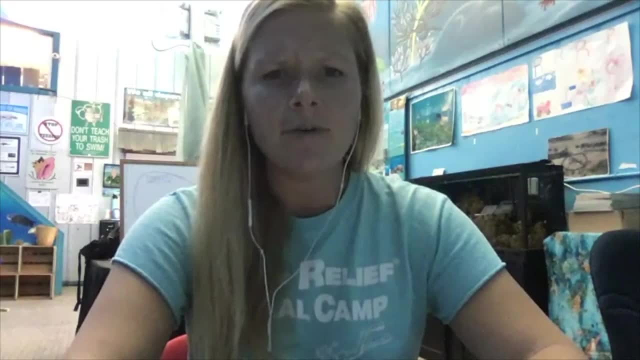 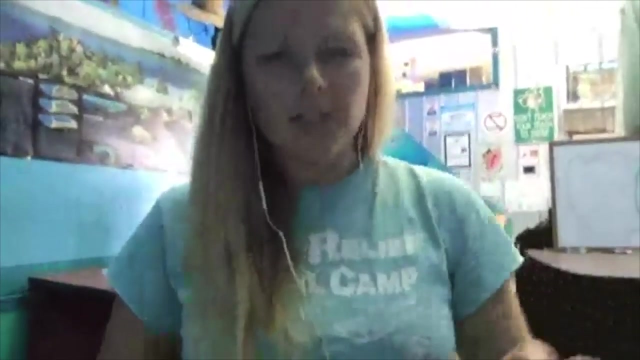 mangroves nearby, So we're kind of found where we find coral reefs. What biome do you think mangroves are found in? Do you think they're found in freshwater biomes or saltwater biomes, so like an ocean? Alright, guys, so good job. It looks like. most of you are getting that correct. Mangroves are found in saltwater ecosystems, And this is actually what makes mangroves so unique. So mangroves, for those of you who do not know, are a plant that has actually adapted to. 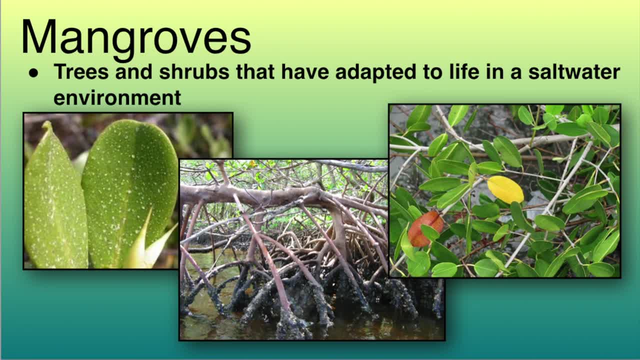 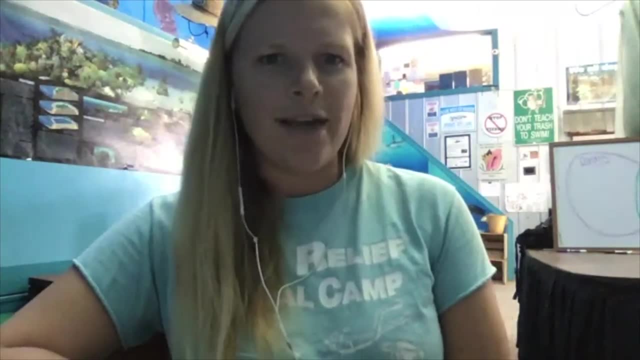 living in saltwater And all that means. that word adapted is just that they have lived and grown into an environment and they have different characteristics that allow them to live in that environment. So let me give you an example really quick. Let's say you go to the store and you 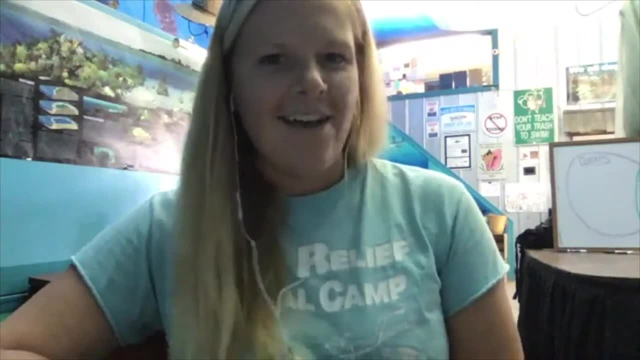 buy some mangroves And you go to the store and you buy some mangroves. And you go to the store and you buy some mangroves. And you go to the store and you buy a bundle of roses for your mom for Mother's Day or for a different holiday. 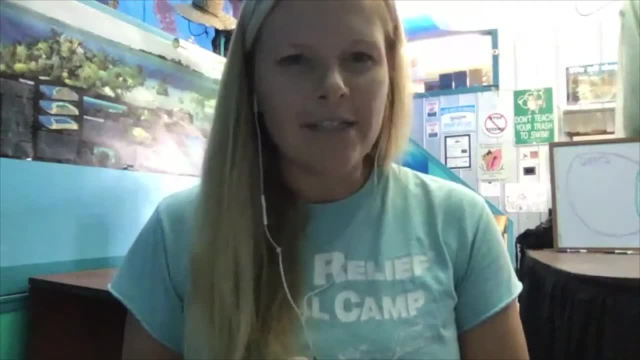 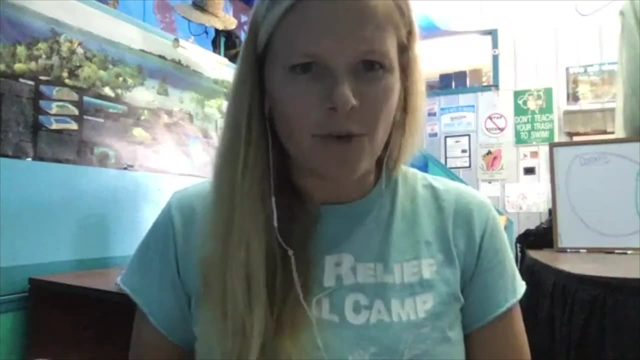 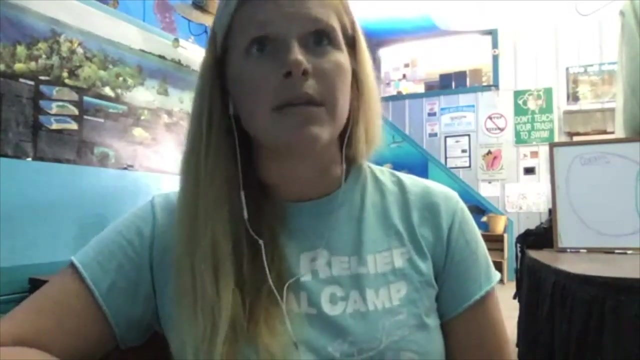 If you have that bundle of roses or flowers, do you guys put those flowers in saltwater or freshwater? You would probably put them in freshwater. If you put them in saltwater, unfortunately, the flowers would probably turn brown, they'd probably get really dry and they probably wouldn't. last very long. Well, mangroves are the complete opposite. They have learned to survive in freshwater or in saltwater, And they suck up that saltwater. they deposit the salt in different ways and then they use the freshwater to live. 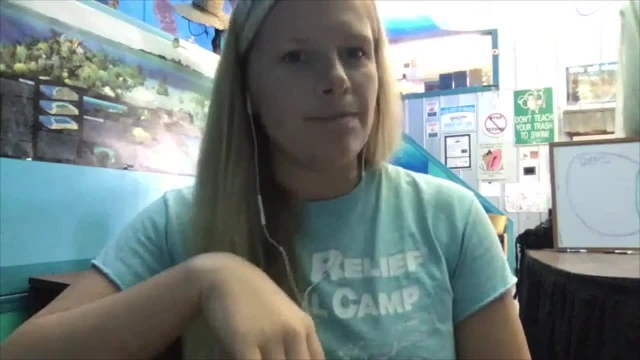 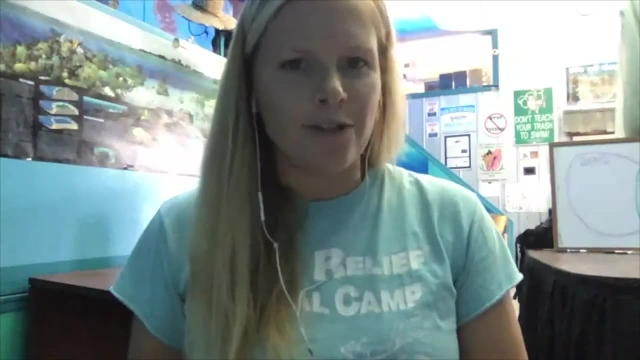 So they are very, very cool, And in a little bit I'm going to show you some pictures of some different types of mangroves that we have in the environment. But first I just wanted to talk about why mangroves are so important, Just like how we were talking about coral reefs being super important. 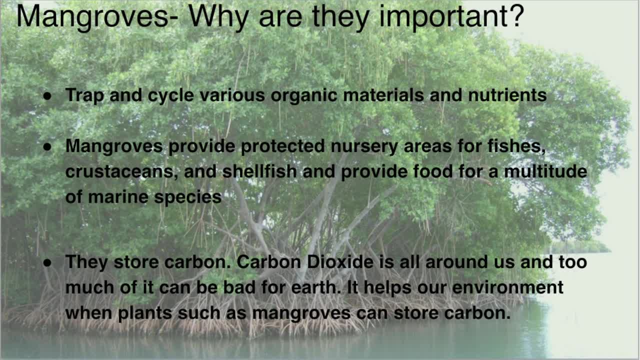 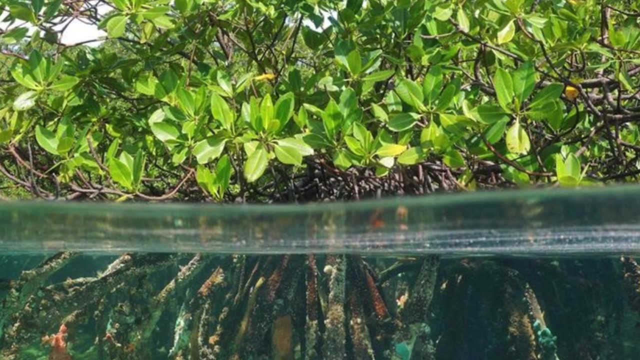 for many, many things. mangroves are as well. The first reason is because they trap dirt and sediment into place to make it not be able to move around, and that helps make the water really, really clear. Let me see if I actually have a picture of what I'm talking about And just like 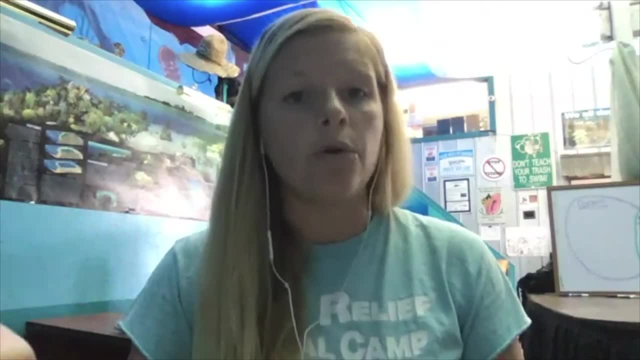 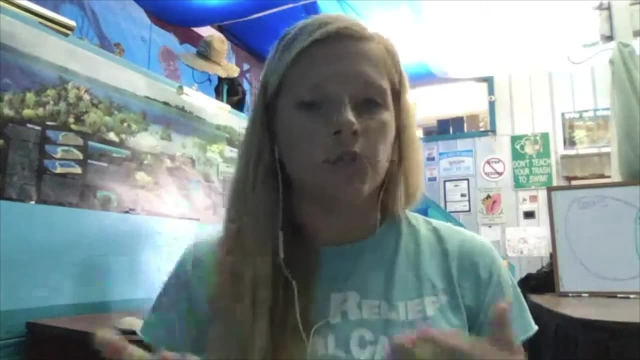 how Miss Dora was talking to you guys the other day about how coral reefs protect from hurricanes and make those waves not as big mangroves do the exact same thing. So let's just do that. Let's do a little bit of a review for a second. So say this hand is those mangrove. 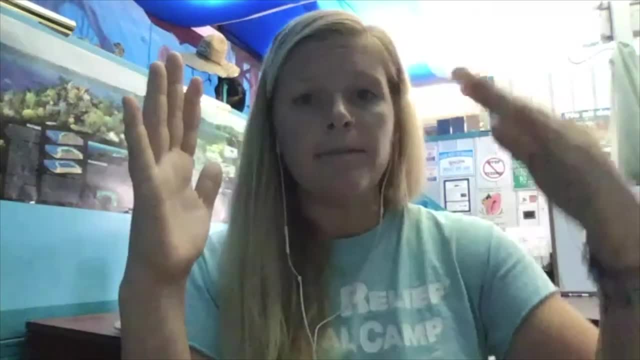 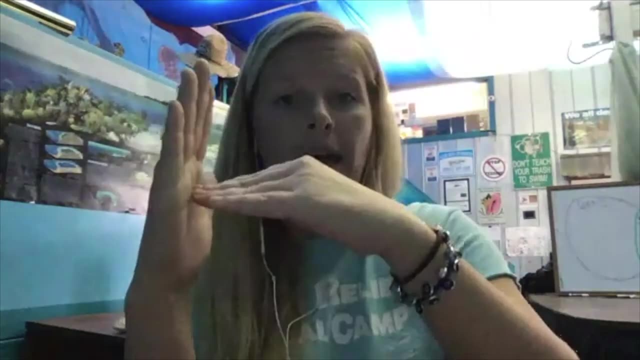 trees that we have, and this hand are some really big waves that are coming into shore. Just like the coral barrier reef, those mangroves are going to act as a barrier to our shore as well from those hurricanes, And so those waves are. 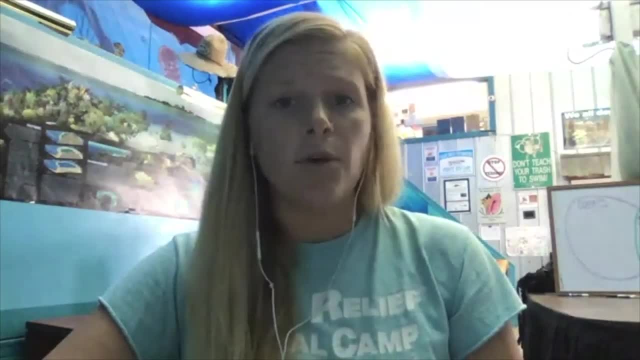 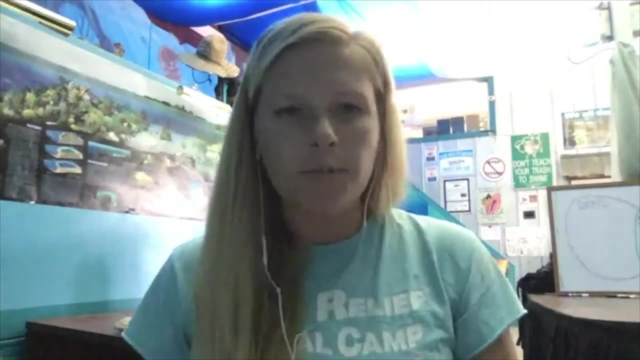 much smaller once they pass our mangroves, So that is awesome for us. They definitely protect us. They're also important because mangroves, just like all other plants and trees, actually store carbon inside of them. Now, I don't know if a lot. 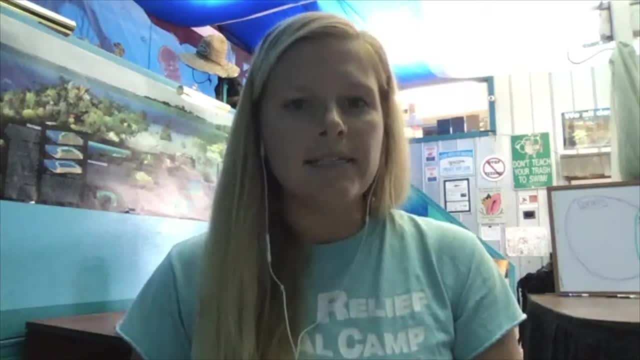 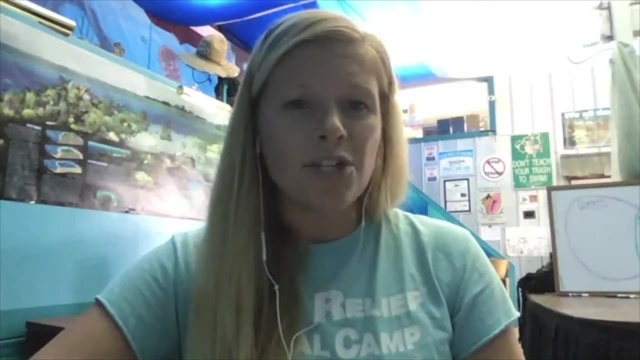 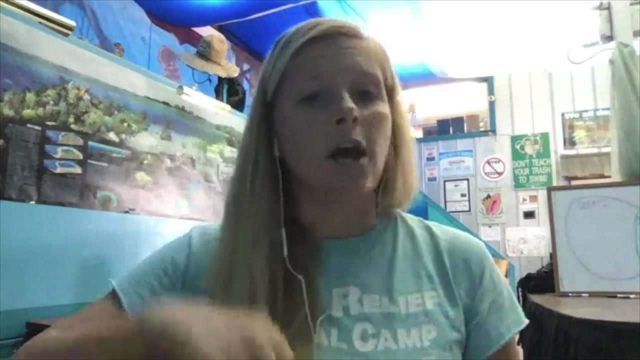 of you guys know what carbon dioxide is, but it is a molecule that we find everywhere on Earth. But the bad thing is that too much carbon can make our Earth really, really sick, And carbon comes from using too much energy so like turning on. 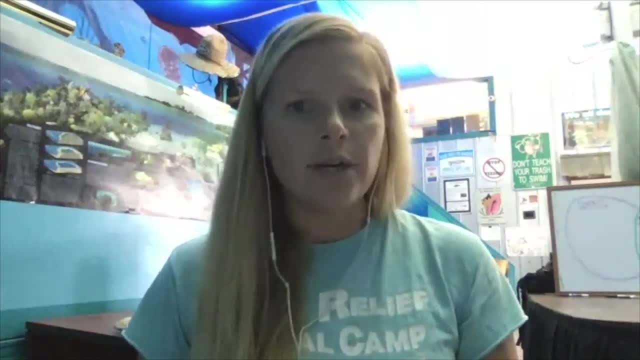 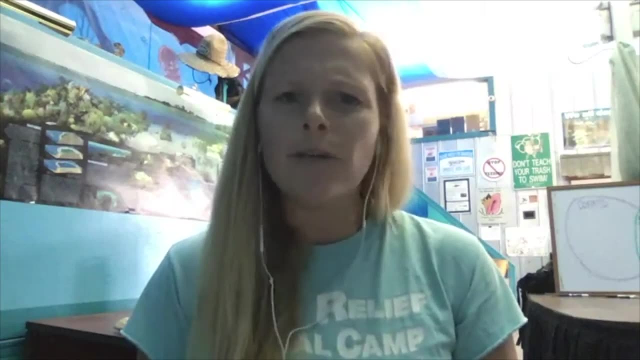 an awful light using a car, anything of that sort- And it's great because mangroves actually soak up a lot of that carbon, or that carbon dioxide, to make sure that we don't have too much of it on Earth, So they're really great for. that as well. So one of the cool things that we can do: just like planting trees, you can also plant these mangroves to suck up more carbon. The third reason of why mangroves are so important is because they act as a nursery for baby. 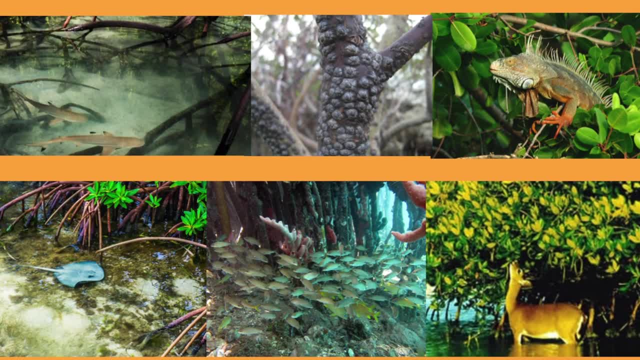 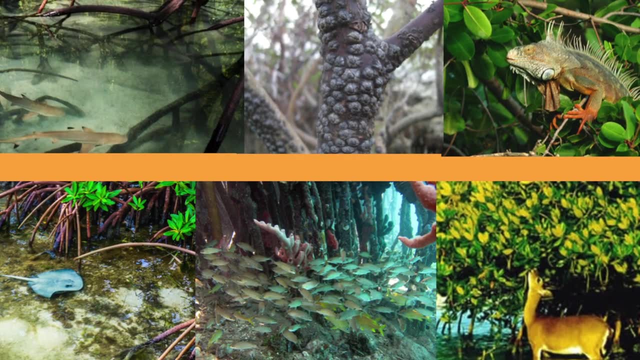 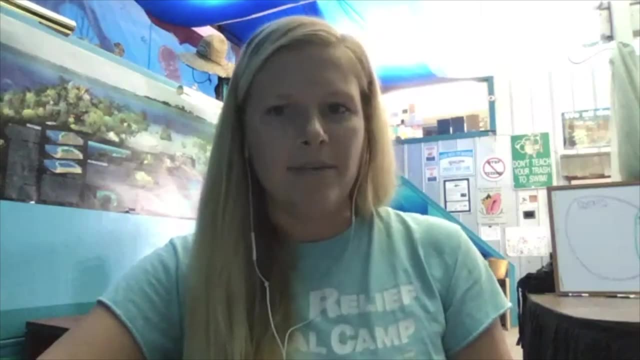 fish. So there are tons of different marine animals that like to make sure that their young are being protected. so, like all their little babies, And a lot of times in order to protect them, they'll take their babies to the mangroves to be able to hide and to be able to grow up in a little bit more of. 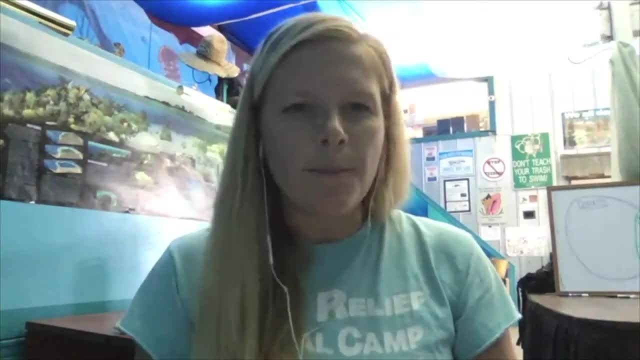 a safe place than a coral reef. Because, think about it, if you were a little baby fish, would you want to be swimming around in the coral reef where there's sharks and huge fish? Or would you want to maybe be under a little tree where there's? 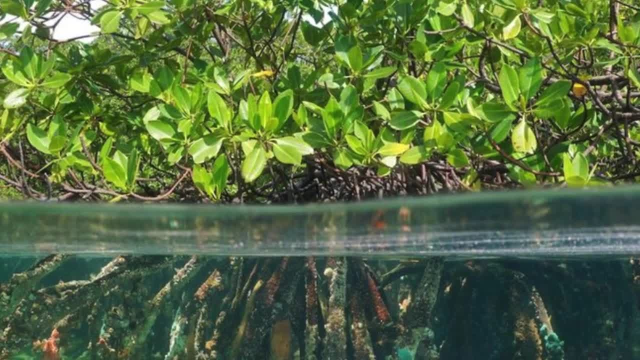 tons of different hiding places. If I were a baby fish, I'd want to be where all the hiding places are. So that's one of the cool things about mangroves is that they're a little bit more safe than other places are. So we're gonna get started on. 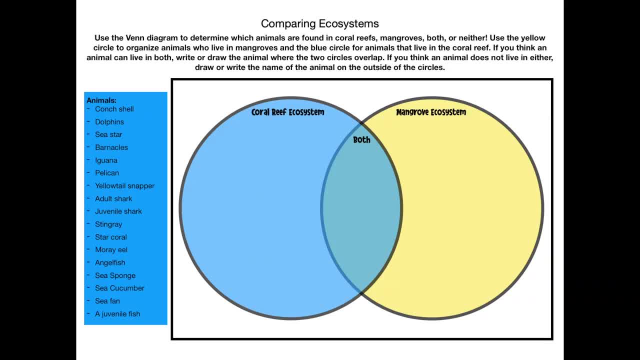 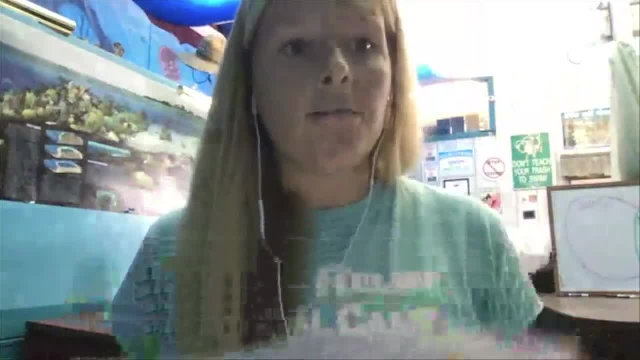 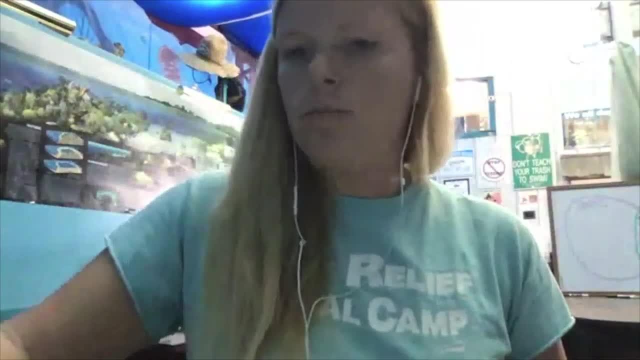 our very first activity. So this is the sheet that I want everyone to take out. We are going to compare our coral reef ecosystem and our mangrove ecosystem together. So everyone take out this Venn diagram sheet right here I'm going to move my computer over. I have also made a Venn diagram on a whiteboard, so 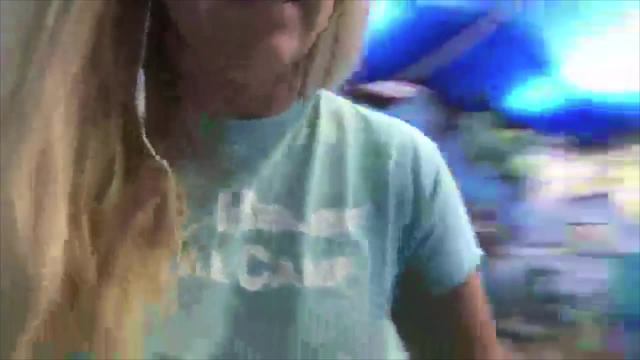 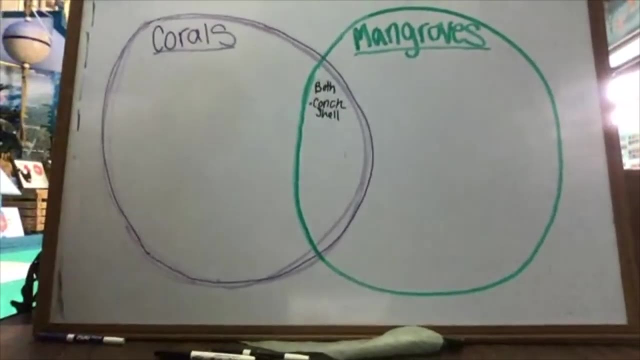 hopefully we can do this together to make it a little bit easier, All righty. so here's my Venn diagram. You guys can see we have corals and mangroves. For those of you who don't know what a Venn diagram is, all it is is it's two circles. 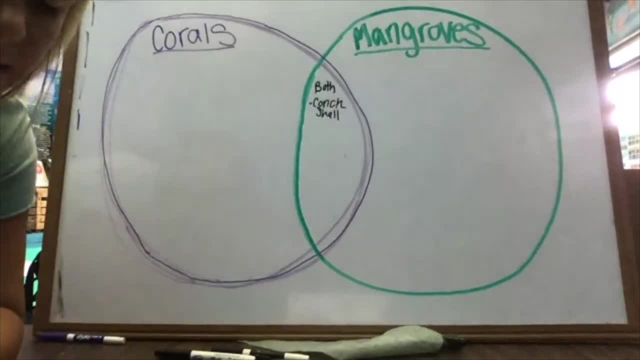 Each have is a label. So for these we're using a mangrove ecosystem and a coral reef ecosystem And it's just how you compare the two. So on your sheet you guys will see your coral reef ecosystem is in blue, Your mangrove ecosystem has a yellow circle And in the middle there's a 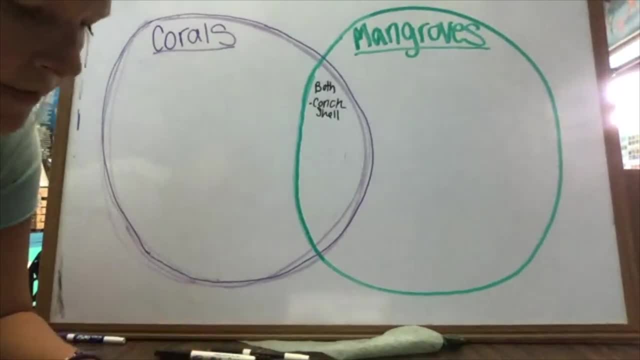 place where they overlap. that's called both Over on the side of your sheet. you're gonna have tons of different animals and we are going to label where each one goes, So the first one I did for us it was a conch shell, So conch. 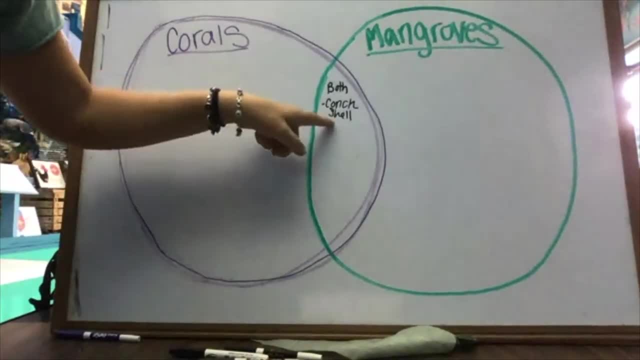 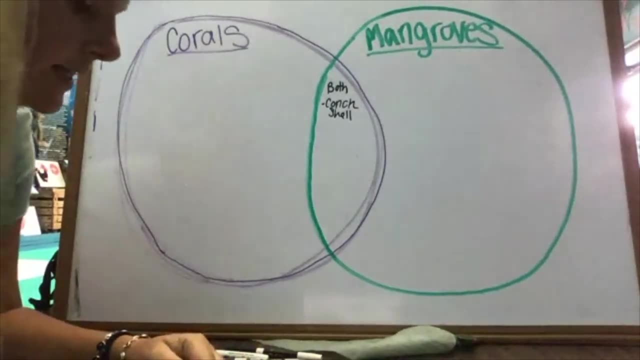 shells would most likely go in the both section, and this is because you can find conch shells in mangroves and coral reefs. So let's go to the next one. The next one is dolphins. So dolphins are pretty big. They probably don't live in mangrove ecosystems just because there's not. 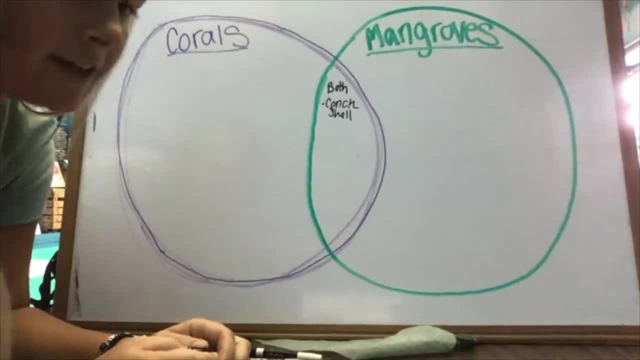 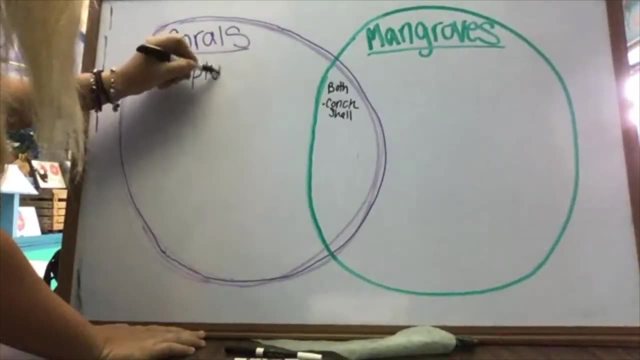 really enough room for them to swim around. So we're probably going to find them in coral reefs. So I'm going to write them in the coral reef section, And just so you know. I'm going to write them. but if you guys prefer to draw the, 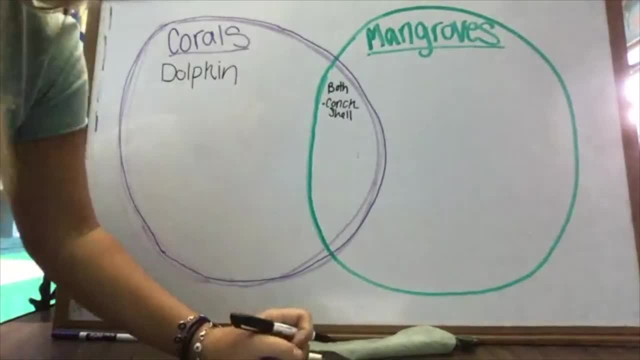 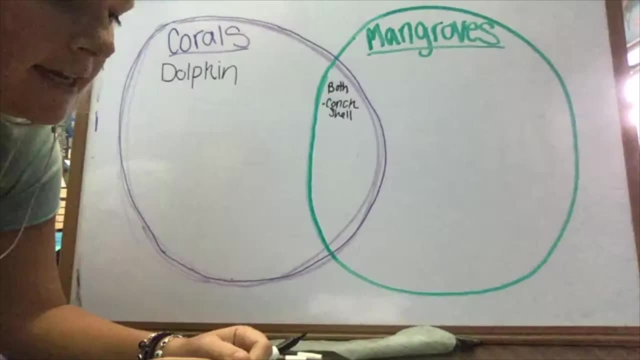 animal. that's totally fine as well. Alright, the next one is a sea star. So sea stars like to live at the bottom of the ocean, kind of in sandy bottoms, and you can probably find them in both. So I'm going to put them in the boat section. 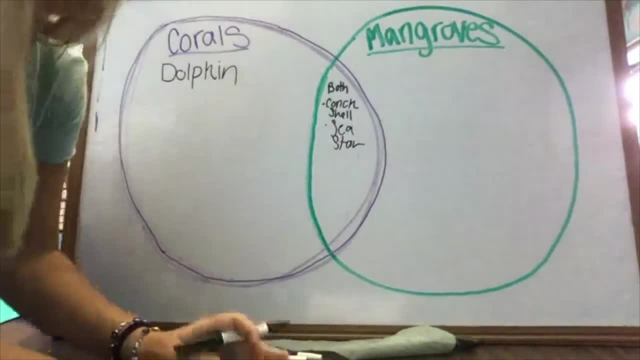 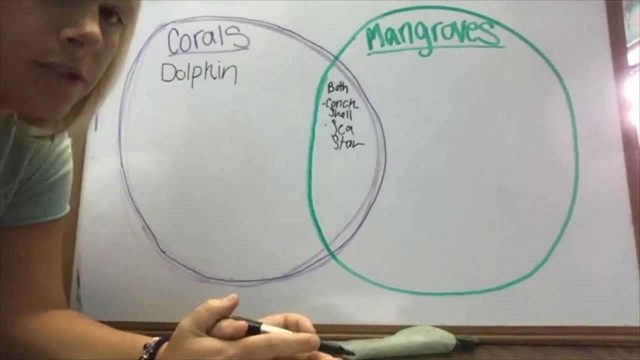 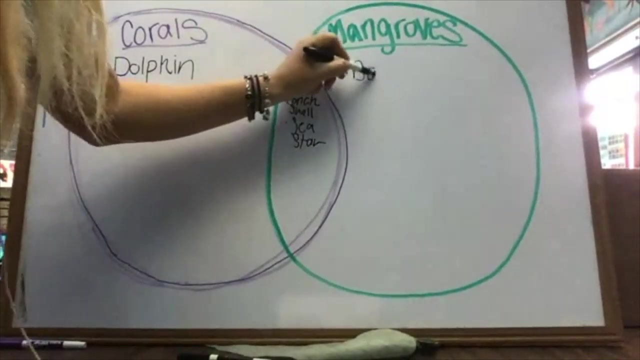 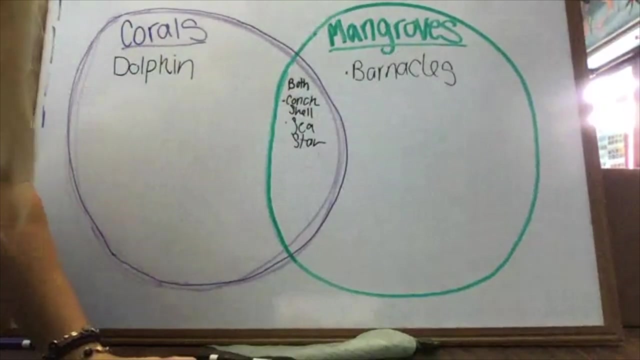 Alright. next up is barnacles. So barnacles are these animals that actually like to live on mangrove roots, So we're going to put those on the mangrove side, Okay, So right here, barnacles. Alright, let's skip around a little bit. After this lesson is over, you guys can. 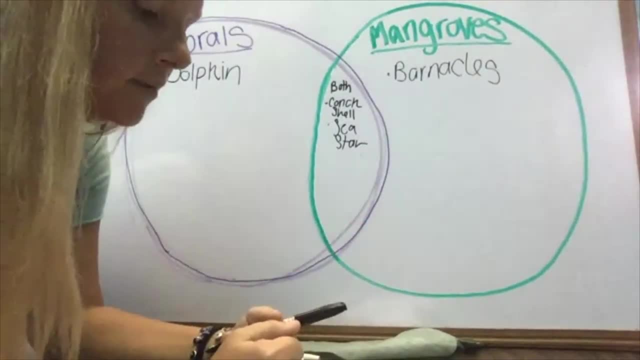 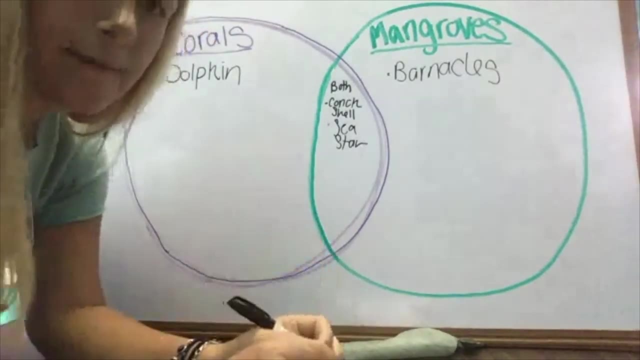 go back and keep adding in all of these animals, But let's just do a few more for an example. So let's go with a stingray. So stingrays are actually a type of fish. They're closer related to mangroves. 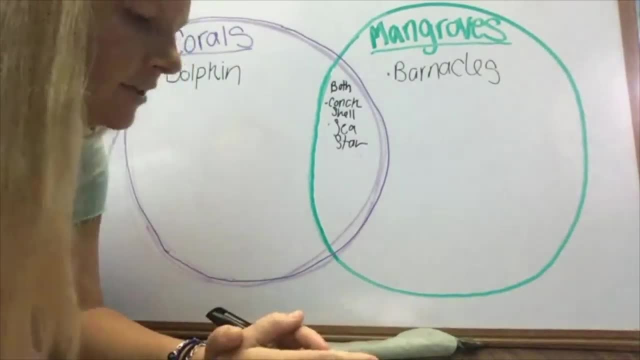 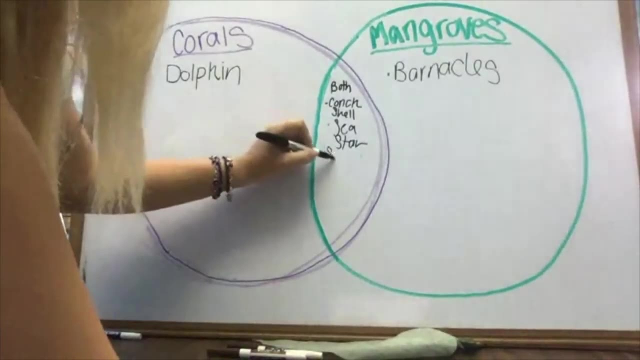 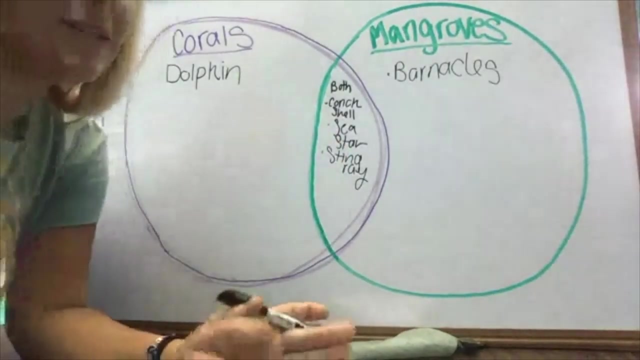 to sharks, though, than bony fish and stingrays. I've seen both at the coral reef and in mangrove ecosystems, so we're gonna put them in both. stingray, all right, I'm gonna give you guys one challenging one. so not every animal in the world fits in these two ecosystems, so where do you guys think you would put? 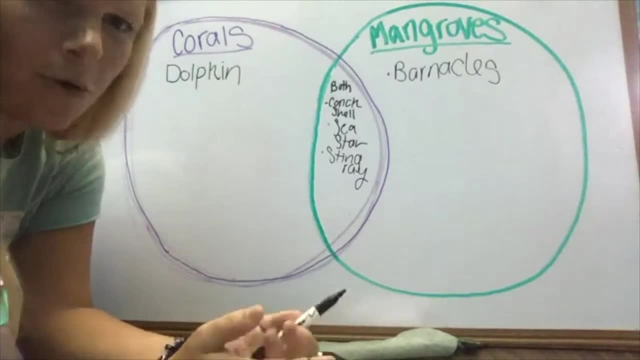 a killer whale. a killer whale or an orca is one of those whales that live in really cold water, so, like the Arctic, pretty deep water. they're really really big. I don't think they live in the coral reef or in the mangrove ecosystem. so if 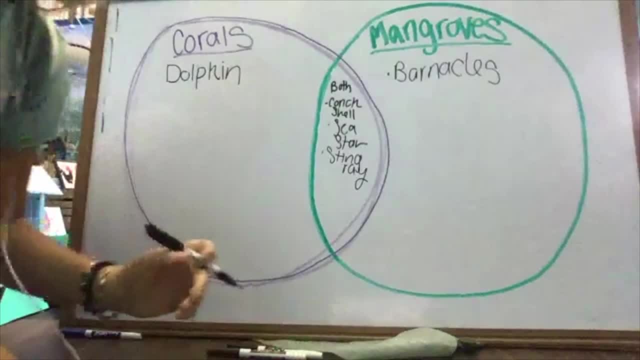 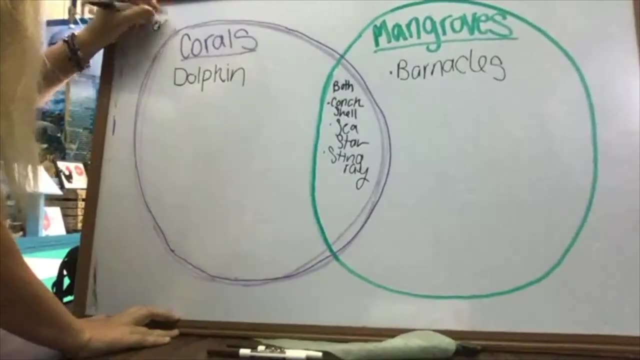 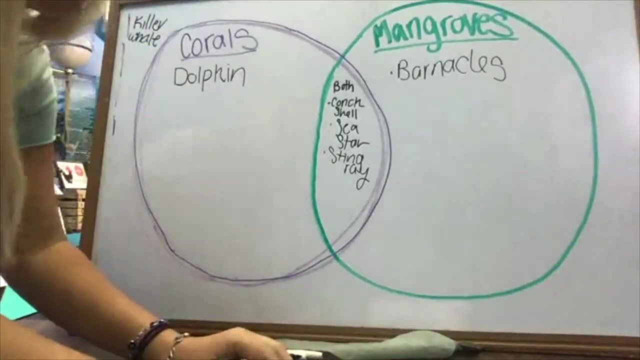 you have an animal that doesn't belong in either of these, you put them on the outside, so we'll put ours right here, killer whale. all right, just like that. and like I said, guys, I'm not going to do the rest. you guys can do this on your own time at home. let's go back over to the desk, you. 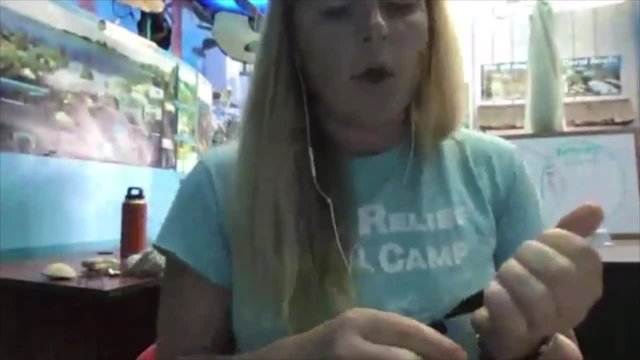 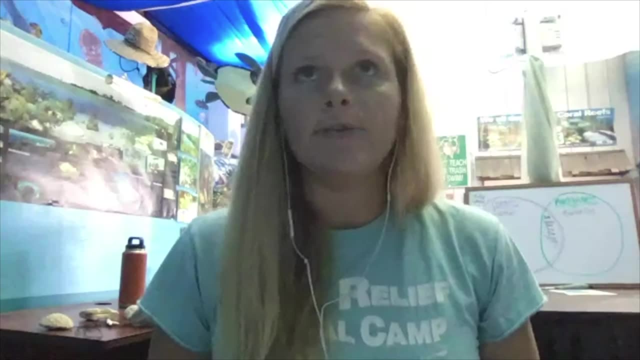 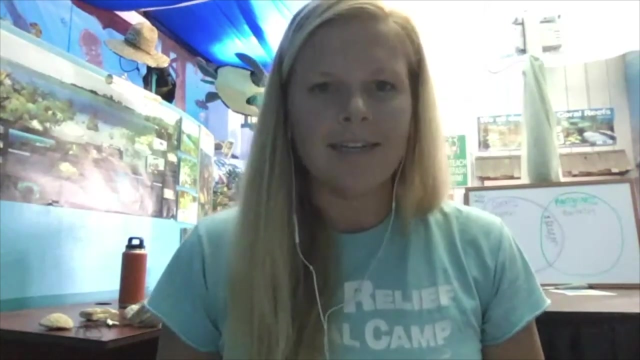 want to take a separate sheet of paper and make your own Venn diagram. you can do those for all sorts of different ecosystems. so if you don't live by the ocean, let's say you live by a lake instead. compare and contrast a lake to the woods or the forest. it'll be really cool to see what animals live in both. 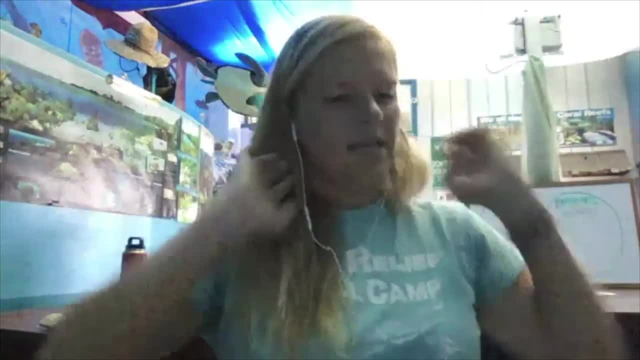 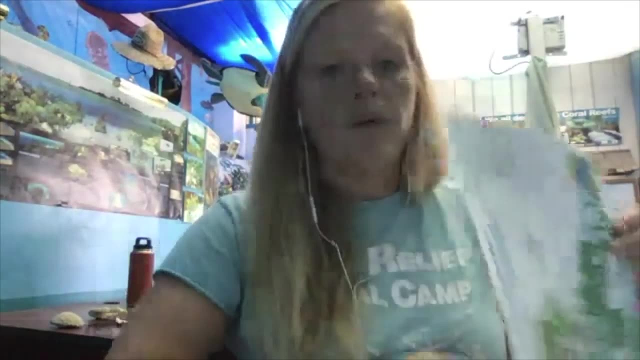 and what animals live around a lake and sometimes live in mountains before live in separate ecosystems. All right, so after the Venn diagram, we are going to directly go to our next activity, which is this marine ecosystems activity. So everyone, get this one out. 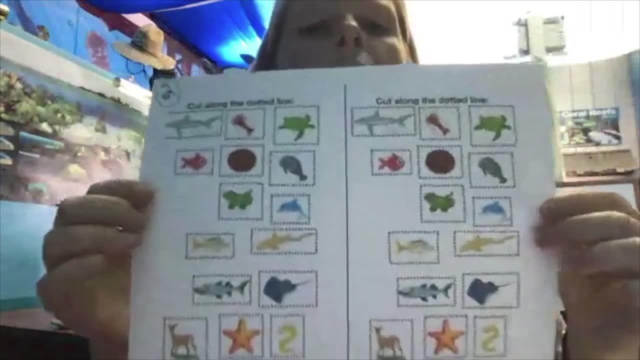 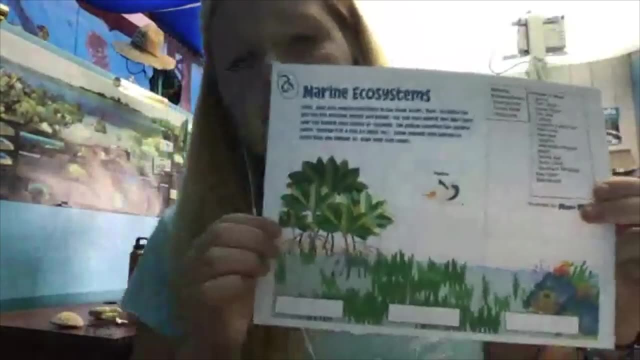 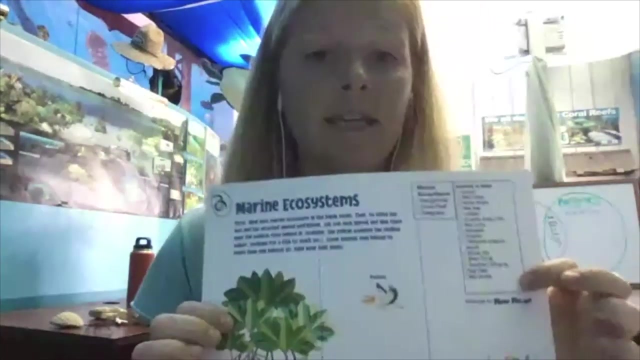 With this, you also have this little cutout. So, guys, a little side note with this marine ecosystems activity is that you'll notice we're going to be talking about mangroves, seagrass beds and coral reefs, So this activity is not going to be finished today. You guys are 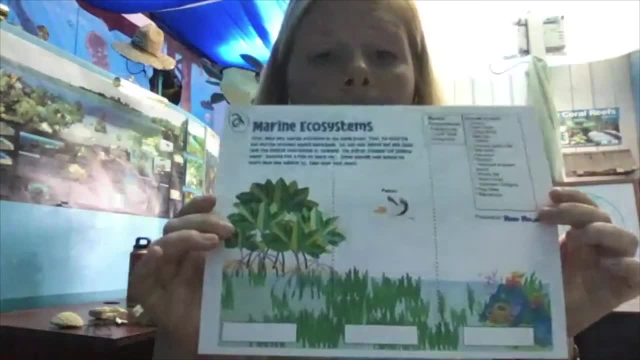 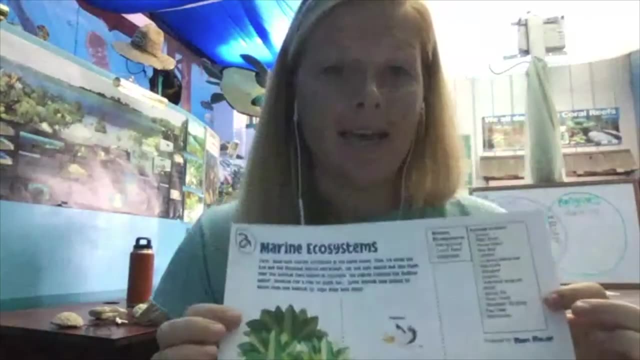 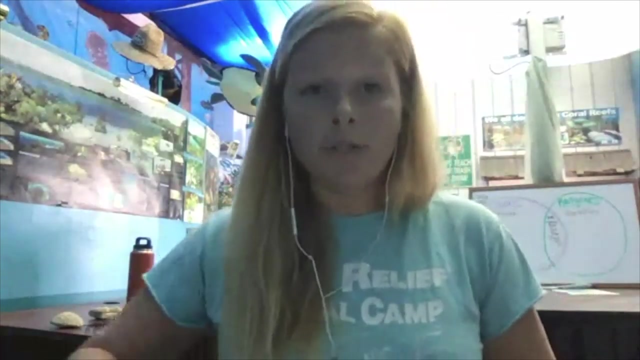 going to finish it on Monday with Miss Dora, because we haven't talked about seagrass yet, and so there's a few different animals that actually live in here. So just do the best you can today, and we will finish it on Monday. Another important thing that I do want to note: 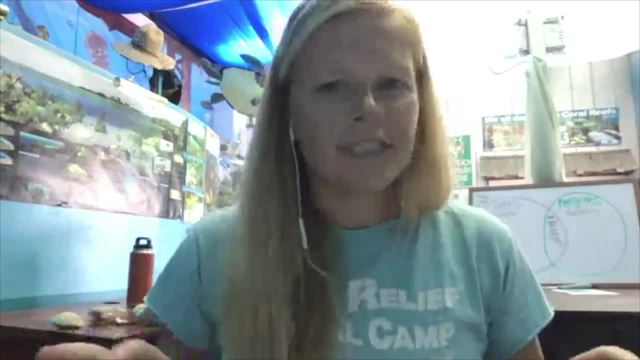 is that not every ecosystem has a perfect path of which to go. So if you're going to be doing a lot of work, you're going to want to make sure that you're doing a lot of work, and you're going to want to make sure that you're doing a lot of work. 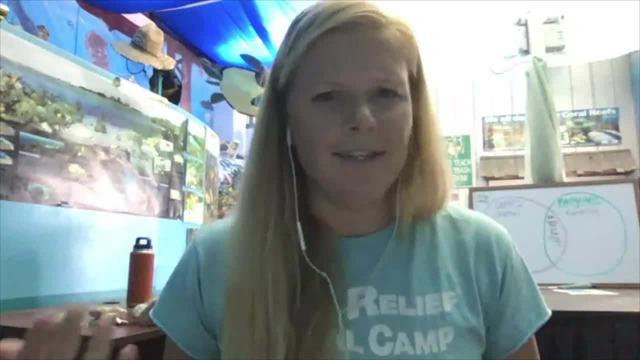 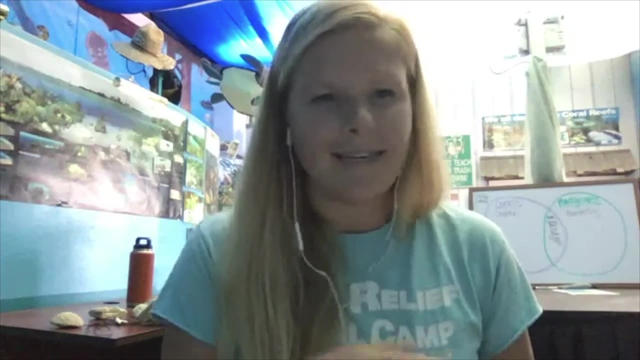 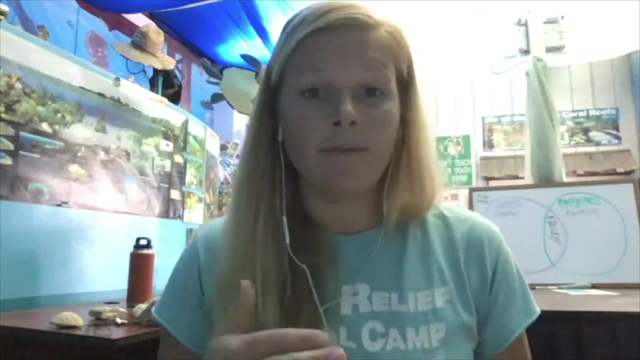 animals live there. There's not roads or gates or fences in the ocean. So just because I think that I wanted to put my fish in a mangrove ecosystem, that doesn't mean it can't live in the seagrass or the coral reef. It can live pretty much wherever it wants to go, but that's just like. 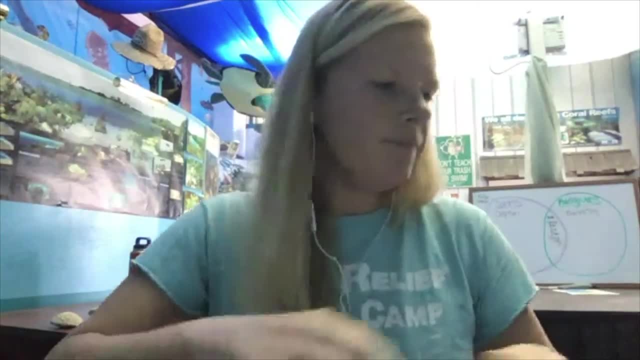 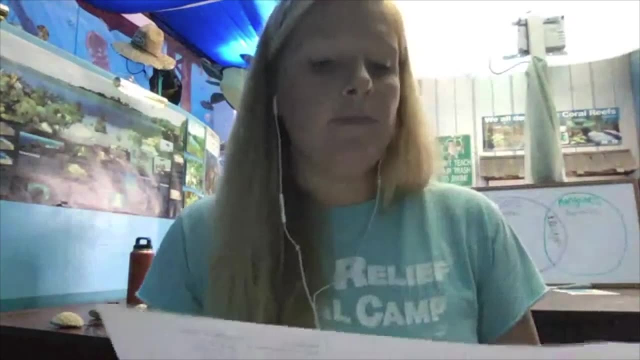 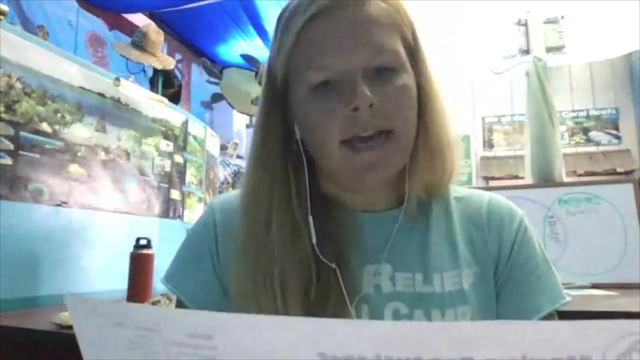 the best habitat for it. All right, so what we're going to do is the marine ecosystems activity says: first label each marine ecosystem in the blank boxes, So you guys see the squares at the bottom. so label your ecosystems Then by using the key attached so that animal worksheet 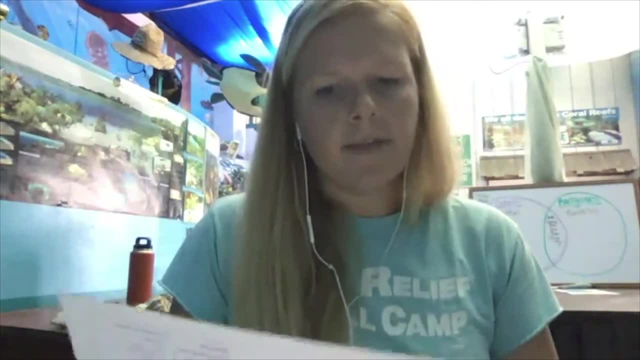 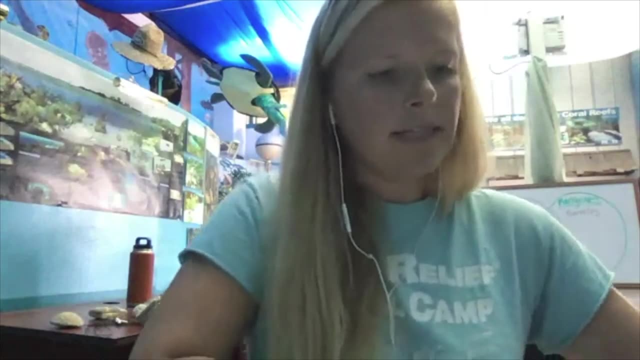 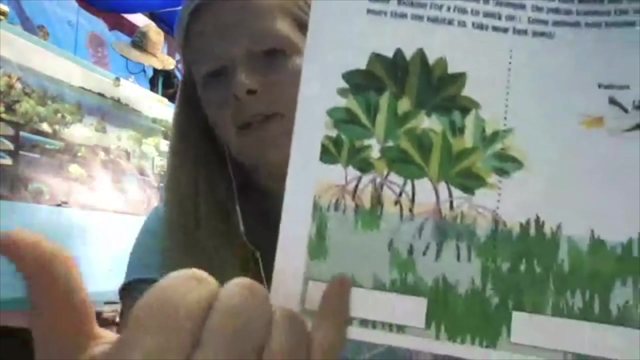 cut out each animal and glue them near the habitat they belong in. Some animals may belong to more than one habitat, so take your best guess. So let's start by labeling. So where those trees are, those are your mangroves, And so see all those roots at the bottom. 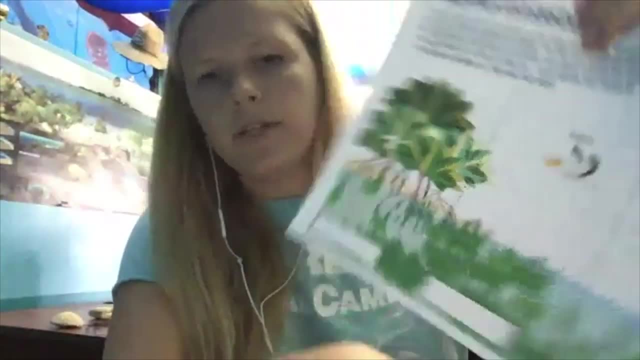 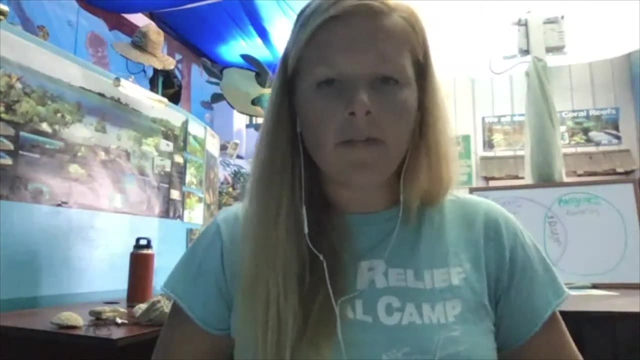 that's what I was talking about a little bit earlier. So that's what a mangrove looks like. So you're going to label in that box mangrove. The next box where all that grass is, that is called seagrass, So you guys can label that for. 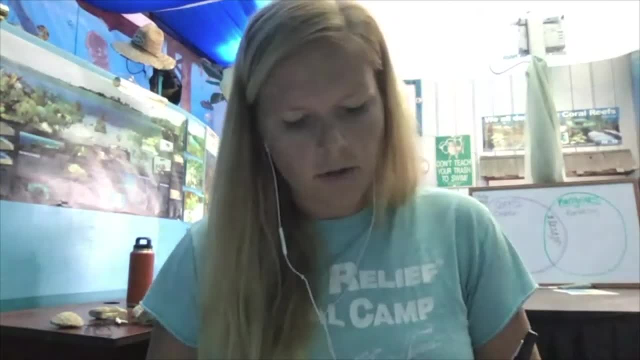 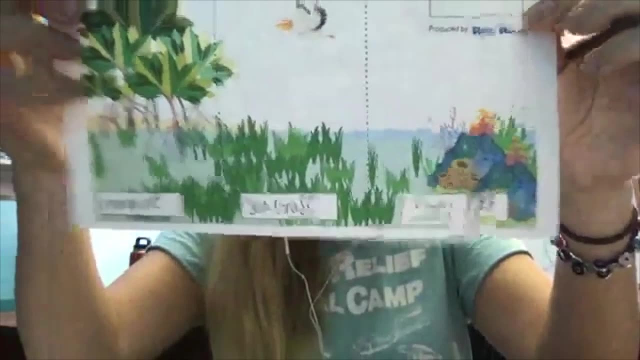 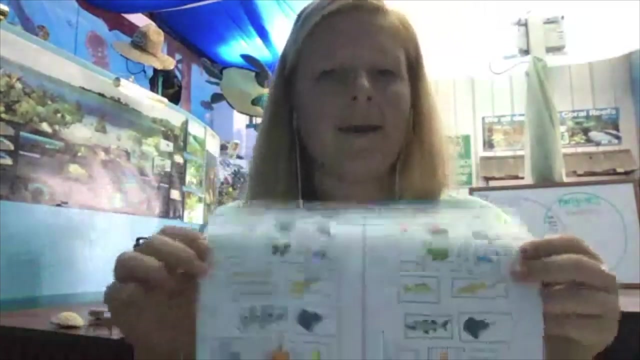 now Seagrass, And the next one is the coral reef. So this is what those three labels are. All right, And next, I'm only going to do this about halfway, because you guys can definitely do this on your own time, It'll. 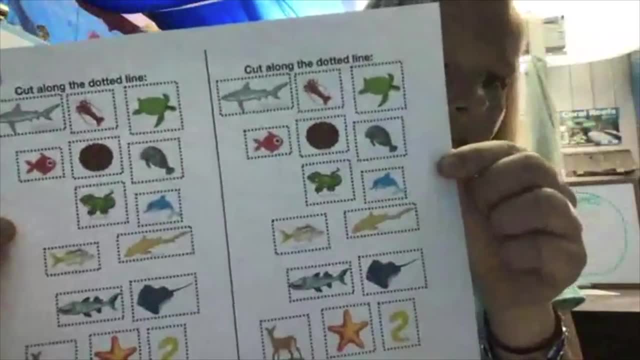 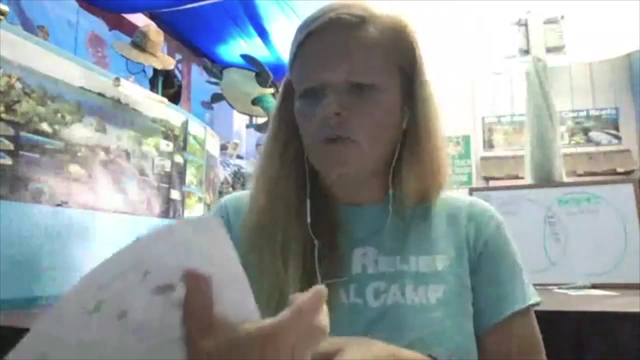 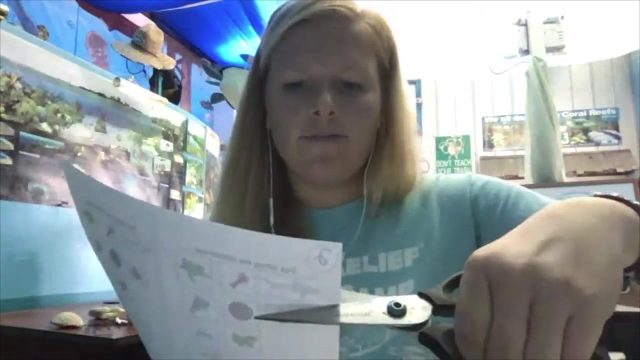 be a really fun activity, But then you're going to cut out each of these animals and stick them on your ecosystem worksheet on where you think they live. So I'll just do one with you guys really quick. Let's do the shark. So the shark is one of the first ones We're going to cut out. the 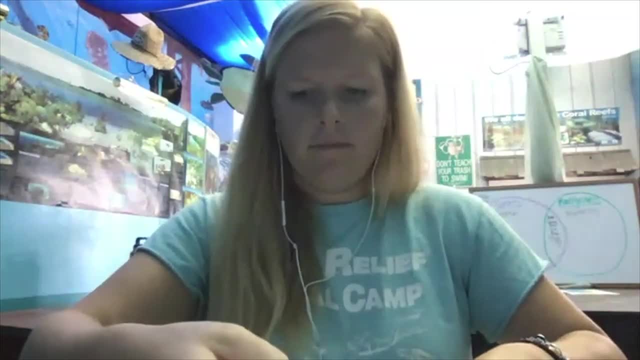 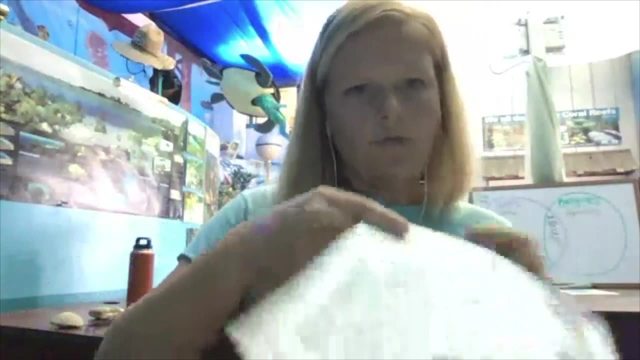 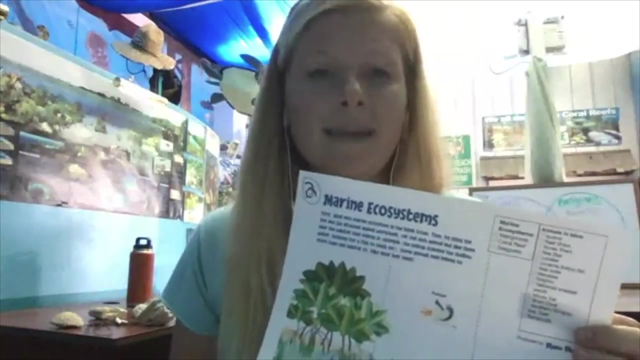 shark Just like this. Here's our little guy And you're going to glue it or tape it to your worksheet. I know that sometimes there's sharks in mangroves, Sometimes there's like baby sharks, And maybe sometimes they're in the seagrass, But this shark is an adult shark, So I'm going to stick. 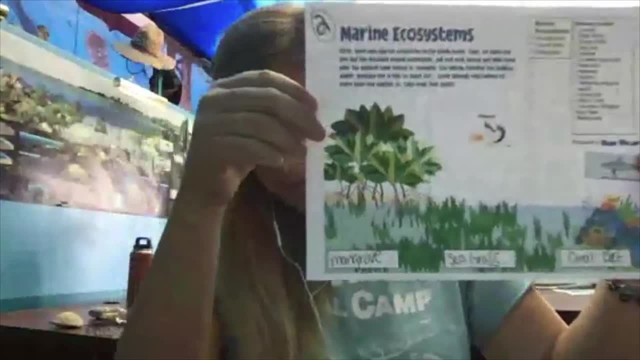 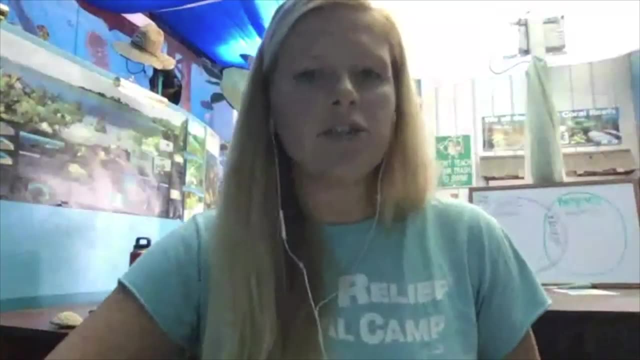 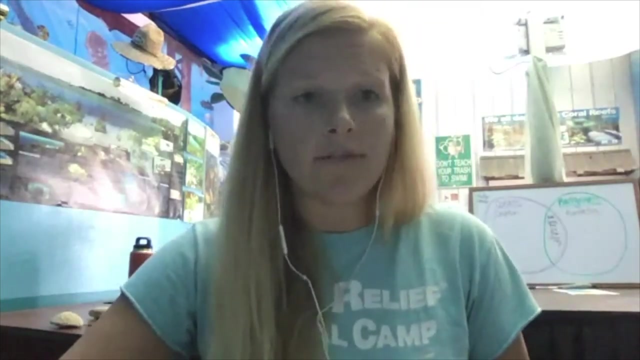 it in my coral reef, Just like that. Let's see. And, like I said, just a reminder, guys, some of these animals you might not know what they are or where they belong, And that's why I'm saying it's totally fine if you don't finish it today. Work on it on Monday with Dora, because she's going. 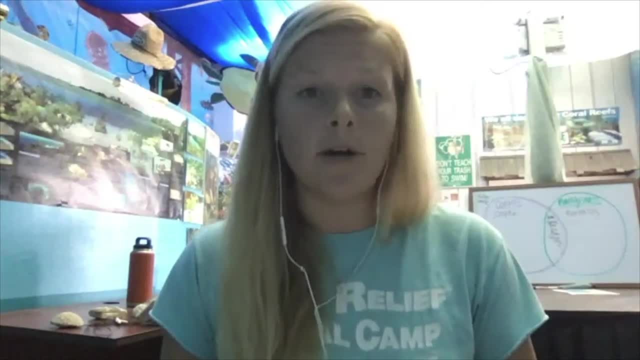 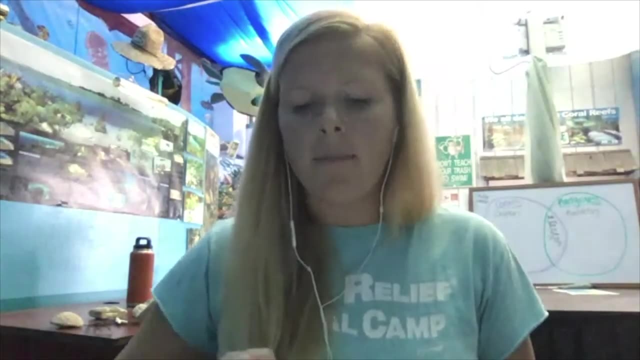 to be able to complete it with you, Because she's going to tell you a little bit more about what lives in seagrass. So actually it might even be a good idea just to cut out everything today and not and place them where you think they belong, but don't glue them yet, And then on. 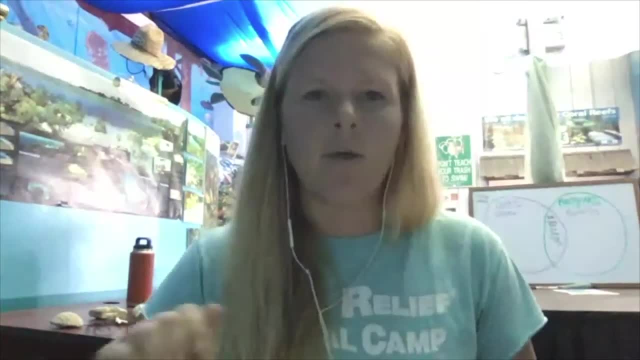 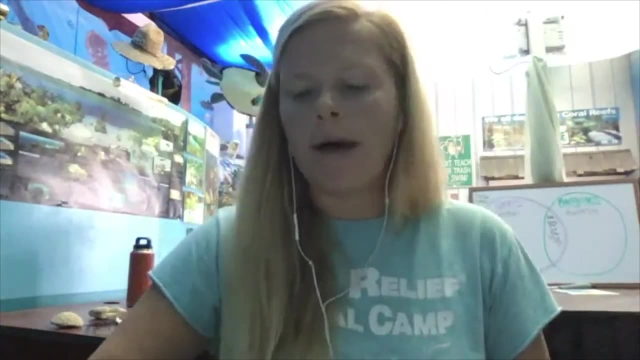 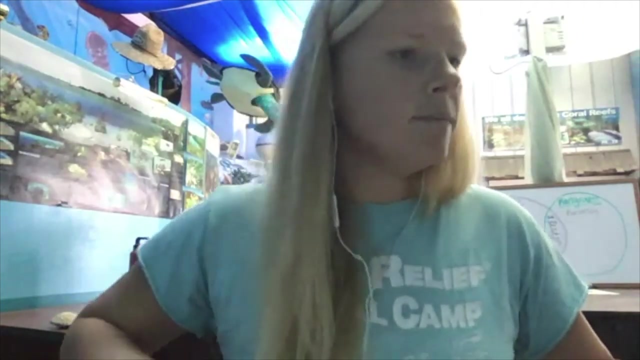 Monday. you can glue them down once you're for sure decided on where you think those animals should go. So that is worksheet number two. So now we're going to actually talk about how mangroves live, what they look like and the different species that we have. So 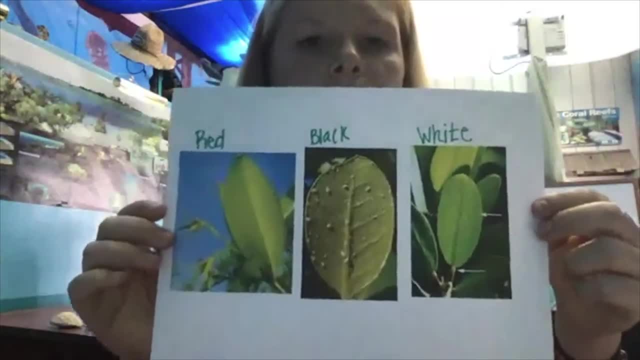 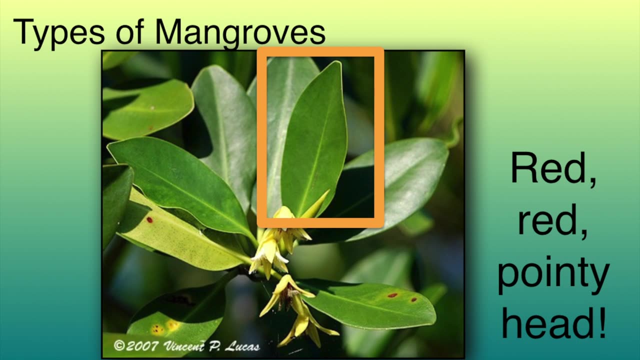 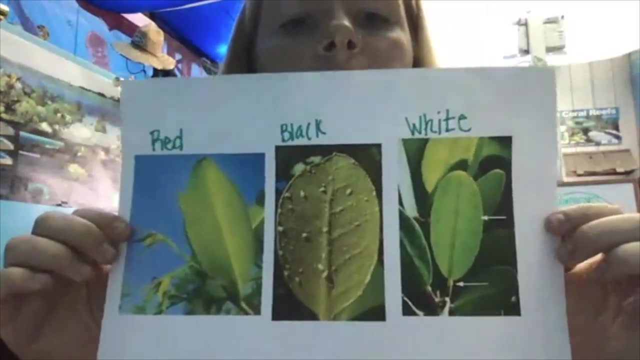 here is a picture of some mangrove leaves. There's three different types of mangroves in the Florida Keys. There are red mangroves, black mangroves and white mangroves, And let me show you this picture again. They all have different leaves And I actually have a rhyme for you guys to remember. 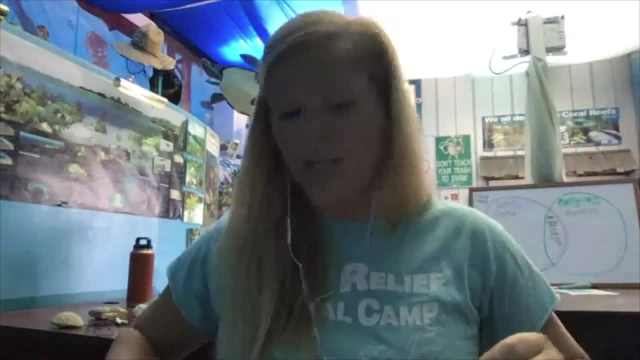 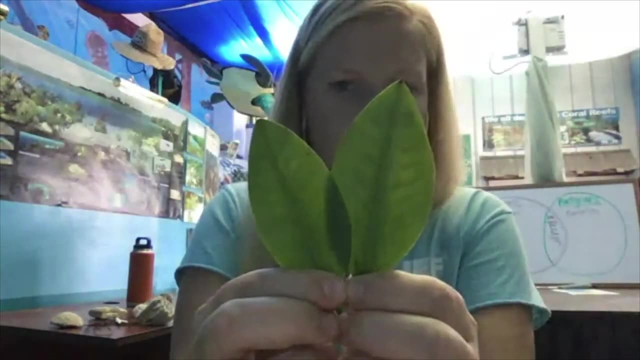 what types of leaves each have. Let me show you some real ones. So I actually went on a little scavenger hunt the other day and found some leaves to show you guys. So these are red mangrove leaves And the way I remember red mangroves is you say: do you guys see how they have like a? 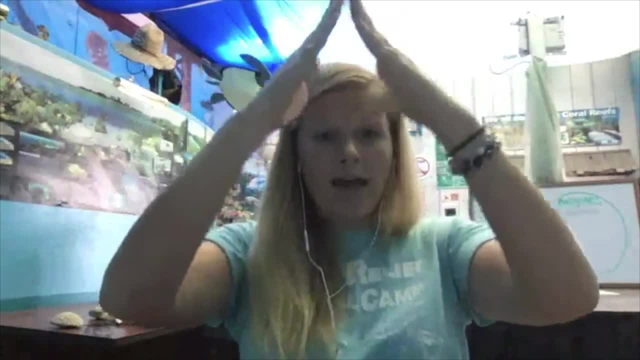 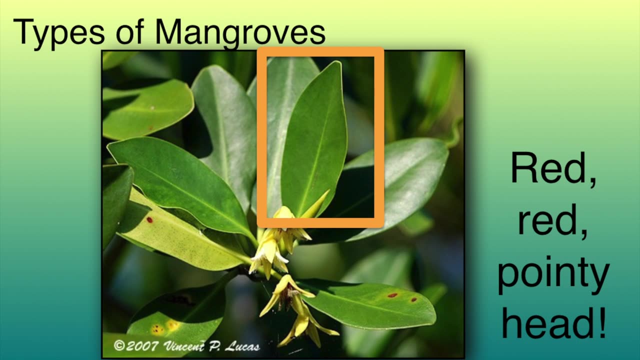 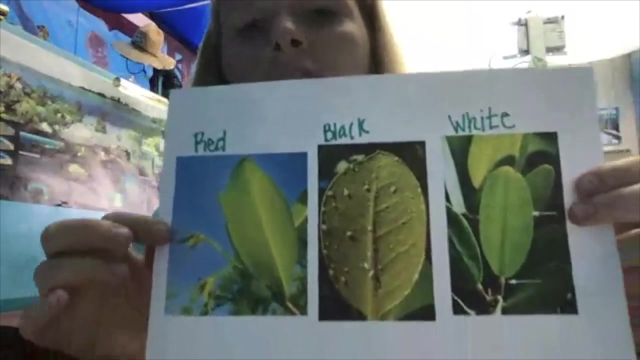 little bit of a point. at the end You say red, red, pointy head. So everyone do that at home: Red, red, pointy head. The next one is our black mangroves And you guys can see in this picture they have little. 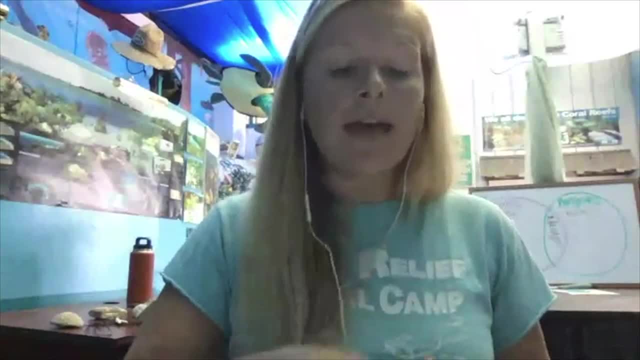 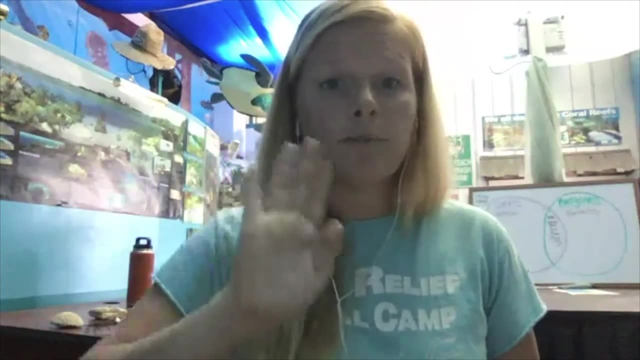 white dots everywhere And that is because that is salt. So, like I said, those mangrove roots suck up all that salt. They have to push it out somewhere. So a lot of mangroves will push the salt off on the backs of their leaves and keep the fresh water to keep living be themselves. 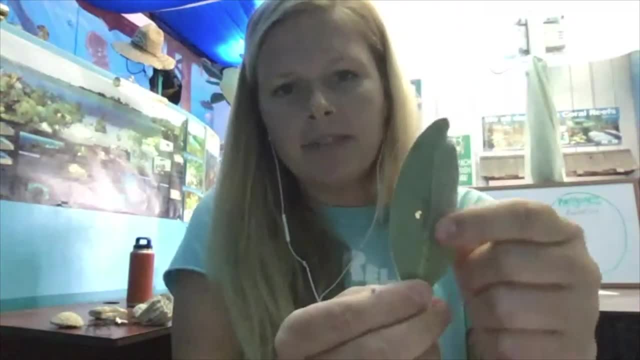 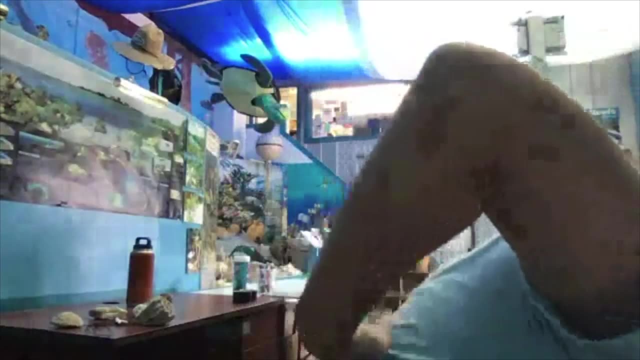 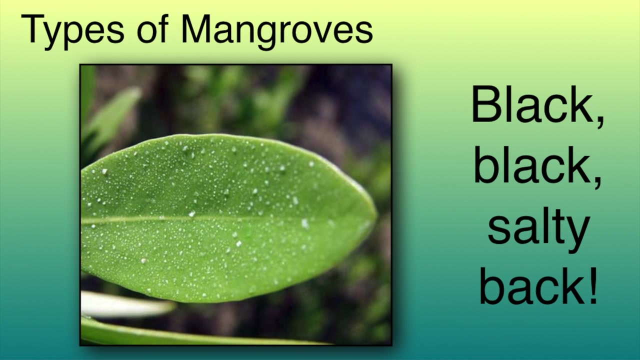 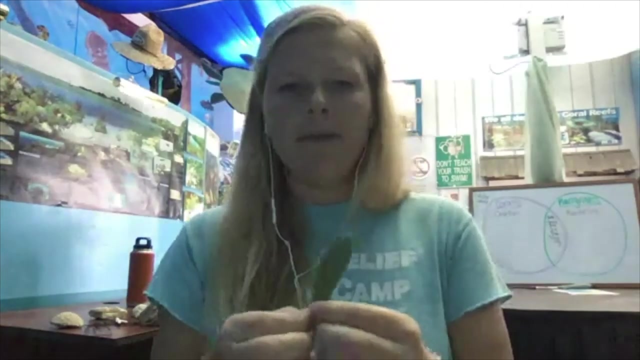 So this is a black mangrove and on the back you can see how it's like a little bit faded and white. that's because that is where all the salt came out of. so you say black, black, salty back. so everyone do that: black, black, salty back, all right. and then finally we have, uh, white mangroves. now white mangroves. look a little. 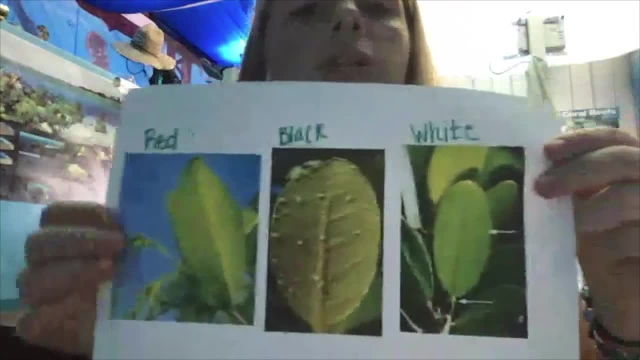 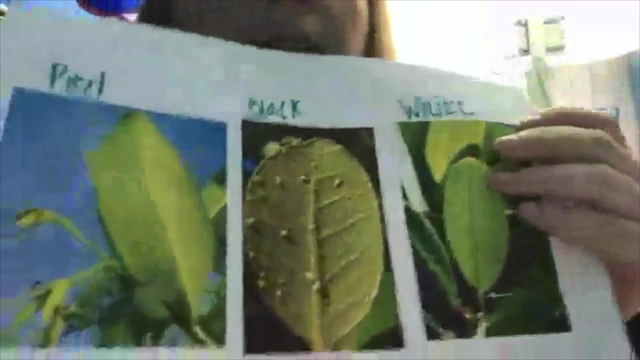 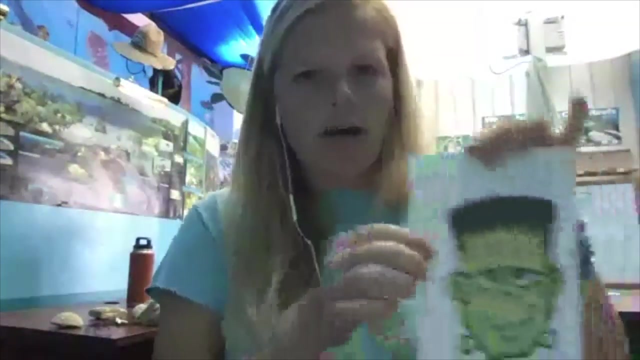 bit like this: um, here is the picture on the sheet, and the way to tell about a white mangrove is: i don't know if you guys can really see, but they have um little bolts on their um stem. so i don't know if you guys know who this guy is. this is frankenstein, but do you guys see how he has bolts? 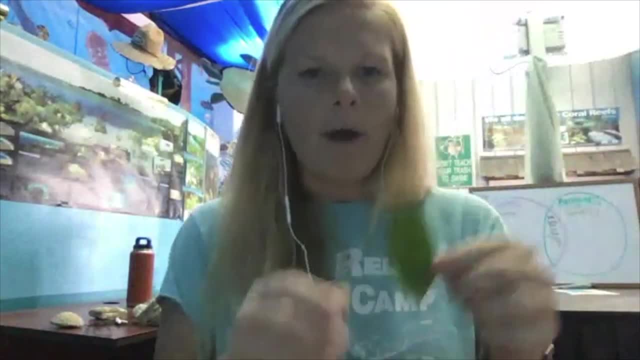 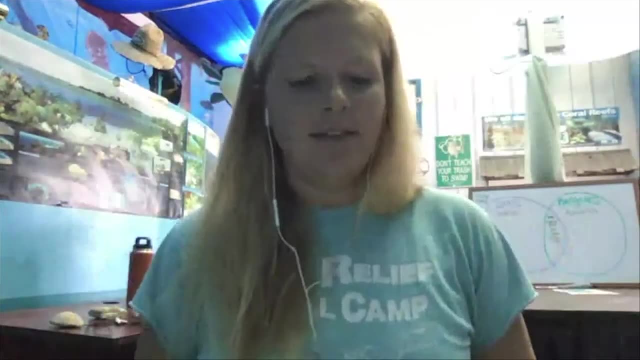 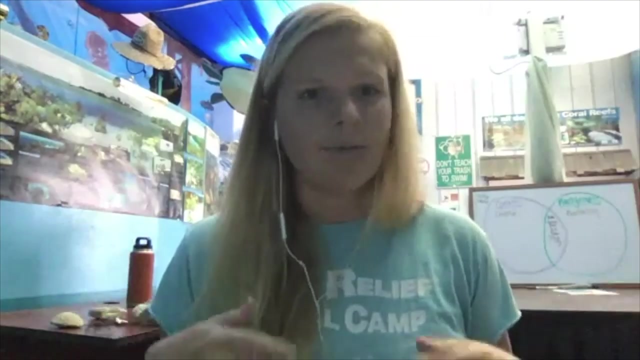 coming out of his neck, so to remember a white mangrove leaf and where these little bolts are right on their stems, you say white, white bolts on tight. so that's how you remember all three. um, so i have a little game for you guys. everyone needs to stand up because we're gonna say this rhyme over and over again. 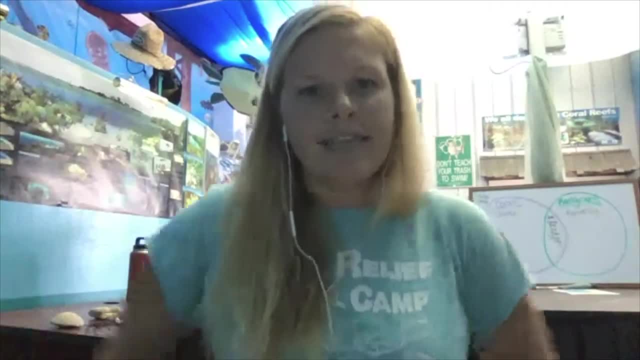 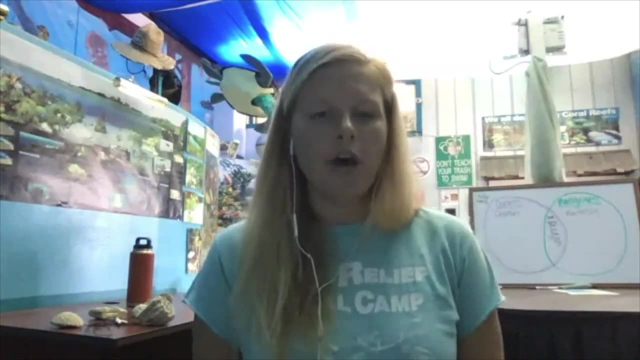 until you guys can remember which species we have, so that once everyone stand up, get a little loose, shake it out a little bit, um, and we are going to uh, do the rhyme over again, so you guys can all remember. so let's do it a little bit slow at first, and then we'll go fast. so red, red pointy head. 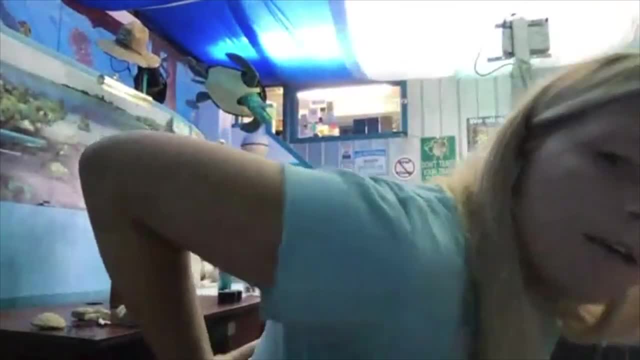 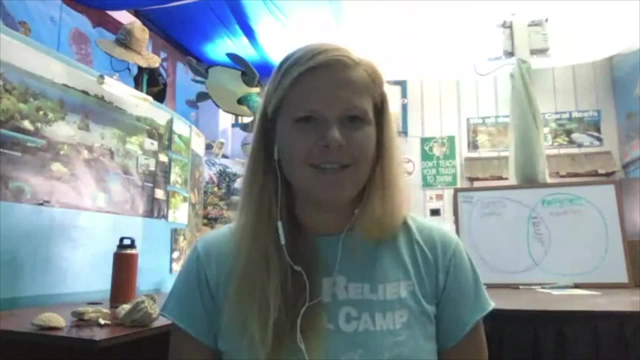 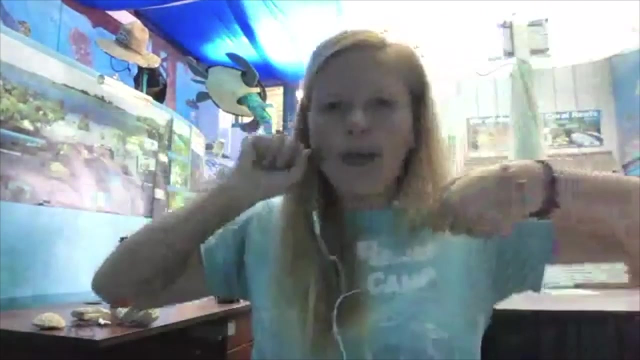 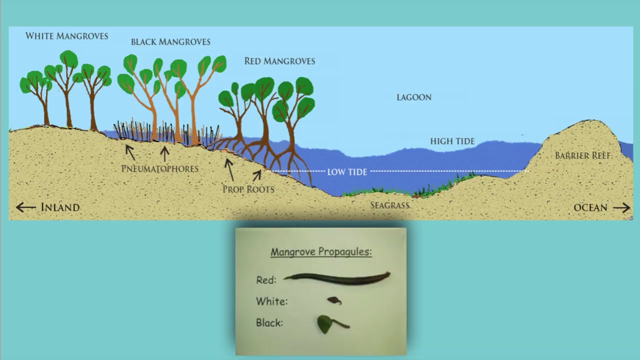 black, black, salty back, white, white bolts on tight. all right, we'll do it a little bit faster this time. so red, red pointy head, black, black, salty back, white, white bolts on tight, all right. so here is another picture. this shows you where all those mangroves we were talking about live. so this first. 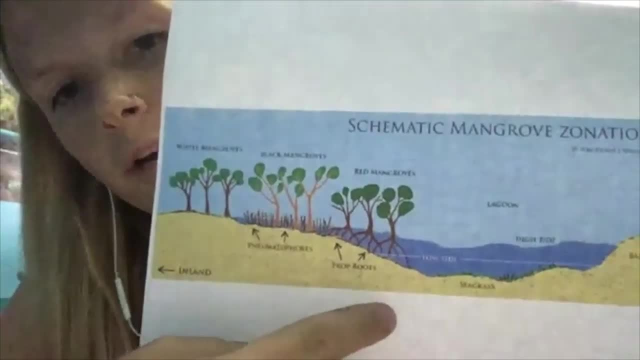 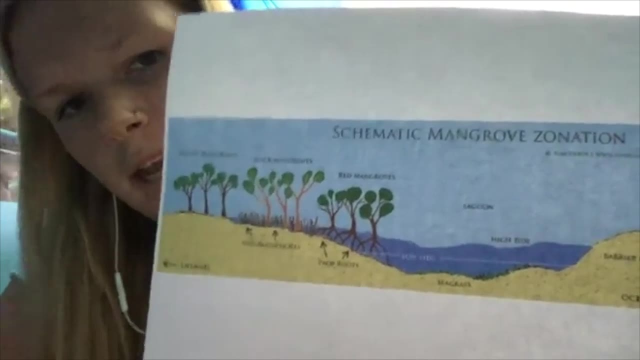 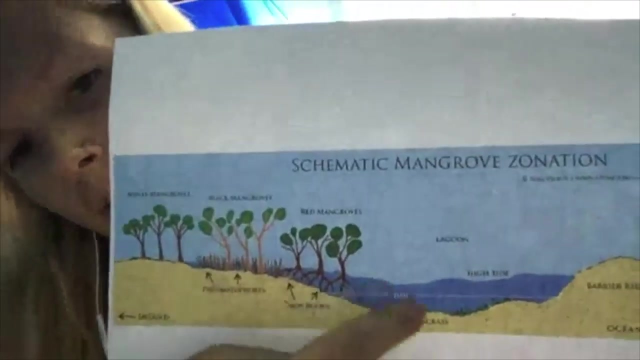 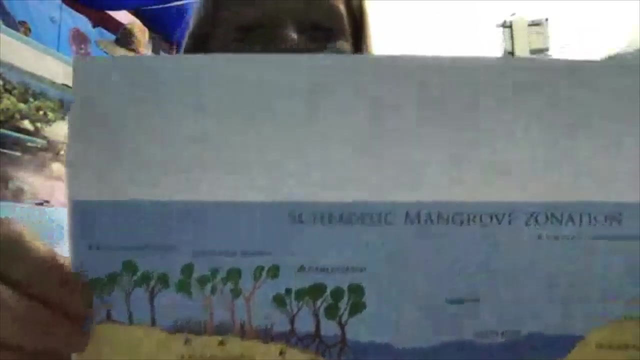 picture shows what some of these plants looked like in living place. so let's do that. all right, there we go. oh, for the year 2000. here it goes. so let's see if you guys can remember each of the matched TWO propagations. community of mangrove- environmentalist. dynamicную soil, inotta human. Those roots for the year 2007 will be ne kannstain, closer to shore or, I'm sorry, closest to the Water. so they have those really big walking roots. those roots are called prop roots. the next will be black mangrove. so we have to see that those roots are sticking up out of the ground. so like see all those thinking up out of the ground. those roots are called Newman. kind of long and hard to say, but basically it just means that they have roots that almost look like snorkels. so if you guys have ever seen a snorkel before, you put it on when you want to go snorkeling or swimming and it helps you breathe. those pneumatophores are those roots. do the exact same thing. they help. 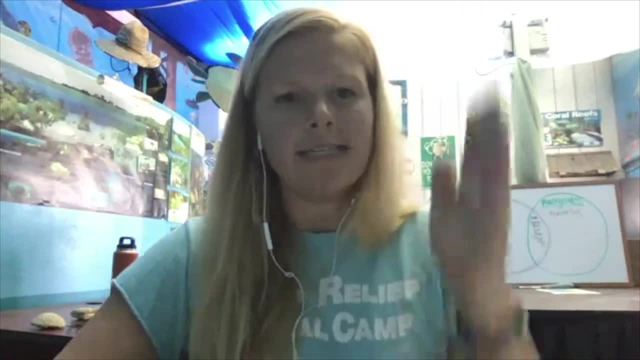 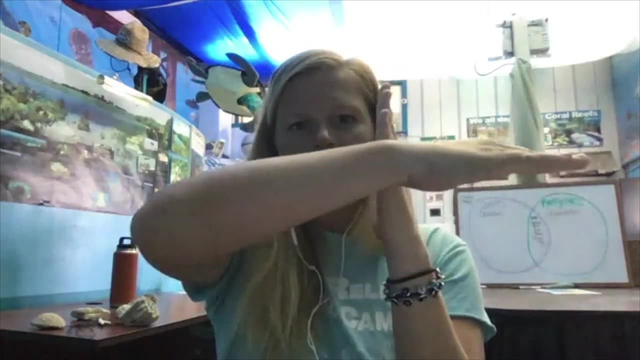 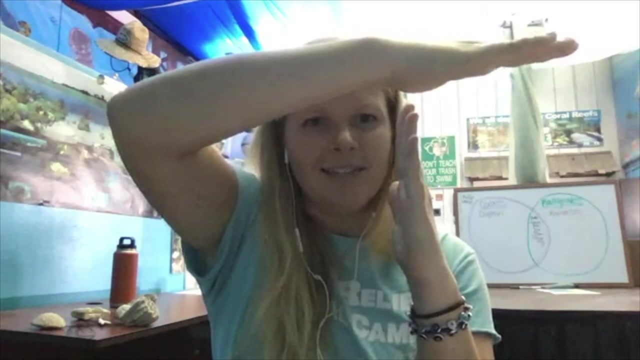 that mangrove breathe, basically. so let's say that this is a pneumatophore right here and this is the tide of the water. so when it gets high tide, the pneumatophore gets submerged completely in water and that's how it feeds and it takes in. 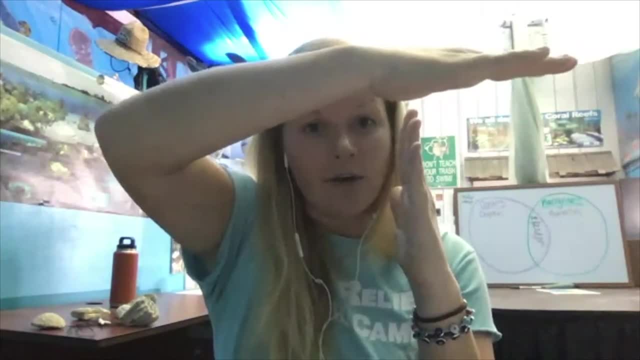 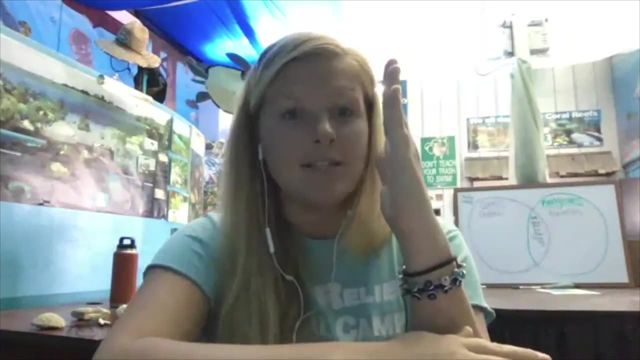 water. but in order to live it also needs air and it also needs to breathe. so when that tide gets lower again, that pneumatophore sticks out in the air and is no longer submerged in water, and it's just a way to help it breathe and live. 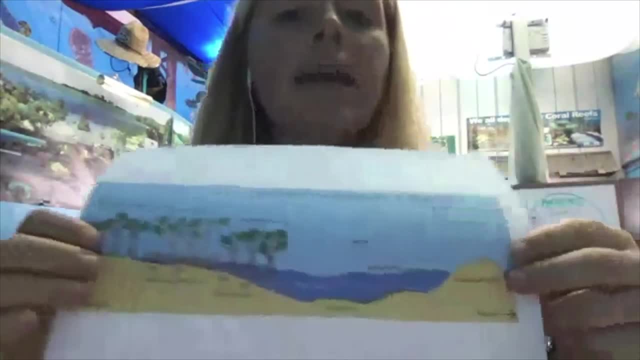 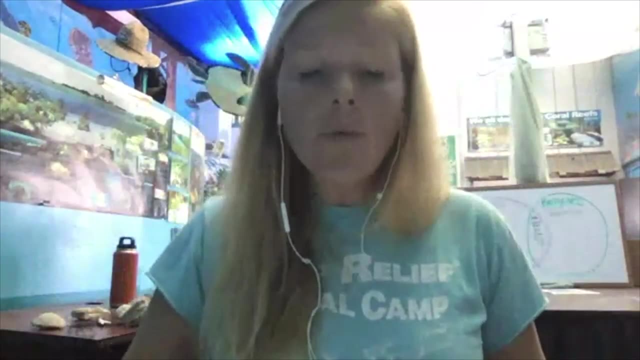 like how it should. finally, on this page, you guys can see farthest away from shore. so right here those are those white mangroves, And although white mangroves still love saltwater, just like its two counterparts, the black and the red, they're a little bit more inshore. They like saltwater, but they don't like to be completely submerged in it. They don't have a good enough root system to be completely in the ocean water, but they still do like saltwater. The last: 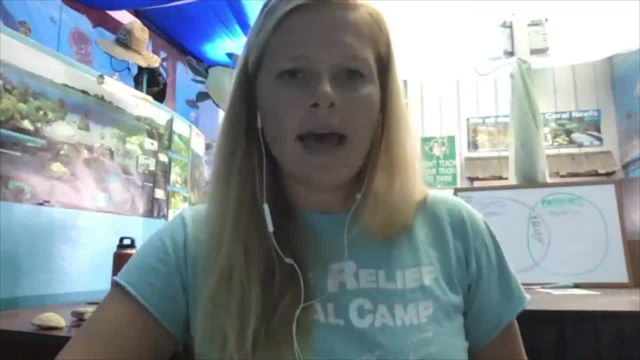 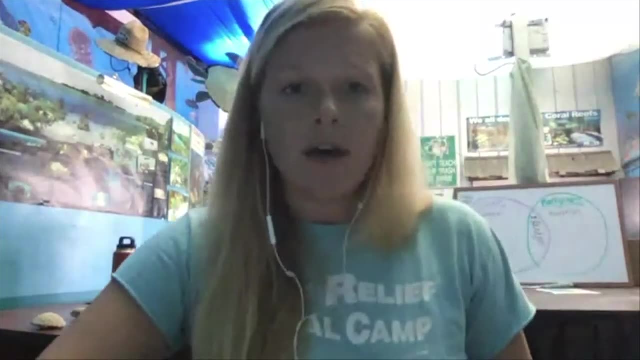 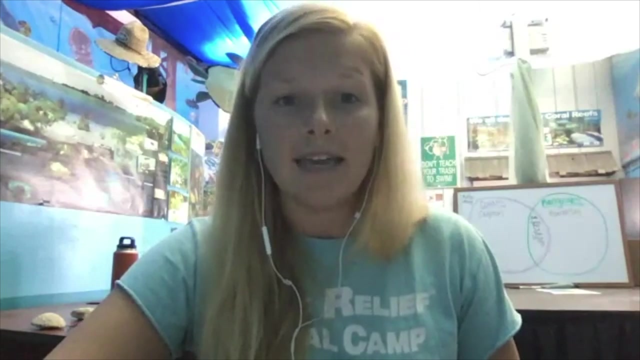 thing that we are going to talk about is how mangroves reproduce and their life cycle. Magroves, like I said, they're unique because they do live in saltwater, but the other reason that they're different from other plants is that they do not have seeds. They have something instead called a propagule, and 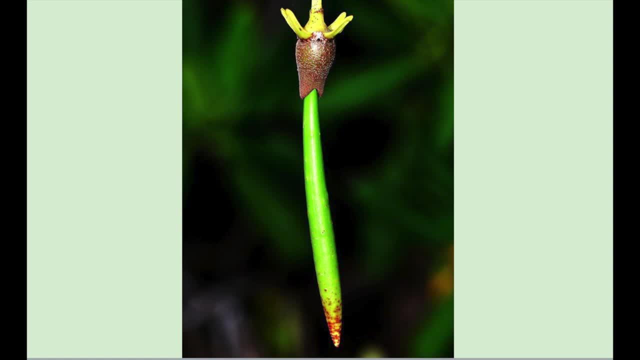 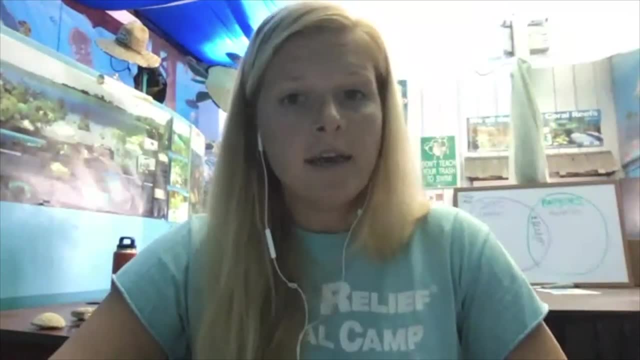 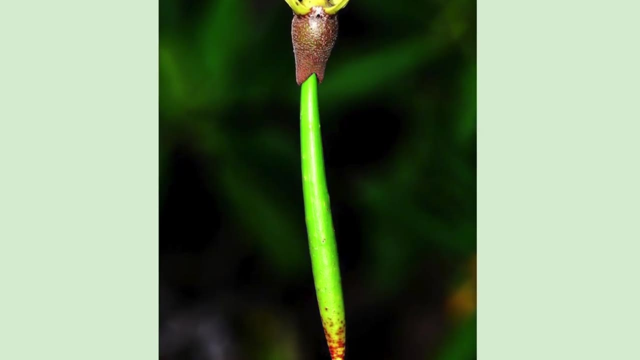 this is what a propagule on a red mangrove looks like. There are those long things that kind of look like string beans. A propagule is different from a seed because while they're still attached to their parent tree, so just like these guys right here, they have already- 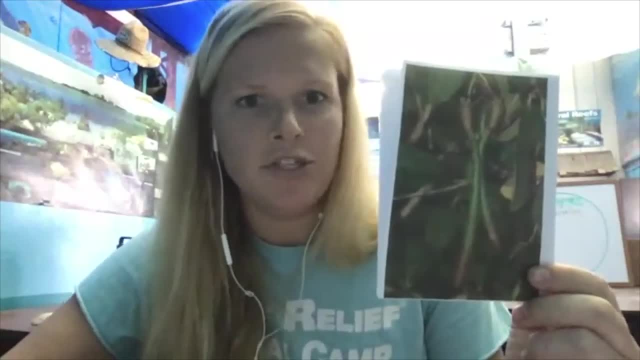 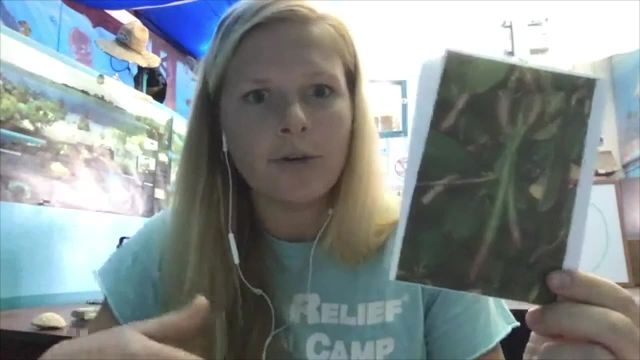 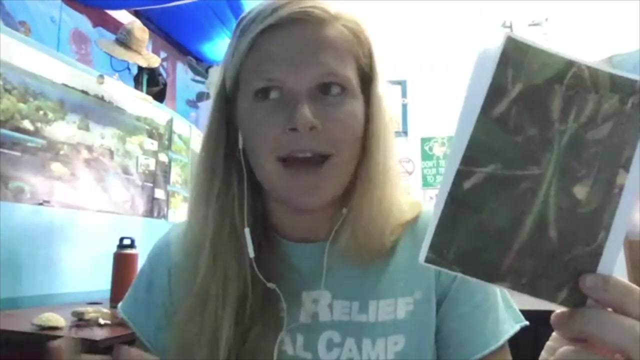 germinated. And germinated just means to be alive and start the growing process, And so these propagules are already like little live babies, while they're still attached to the parents. And this is weird because this is something that other animals do too: They have live birth, so it's very weird to think of a 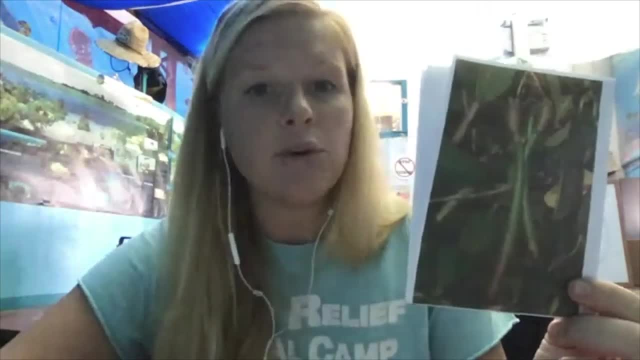 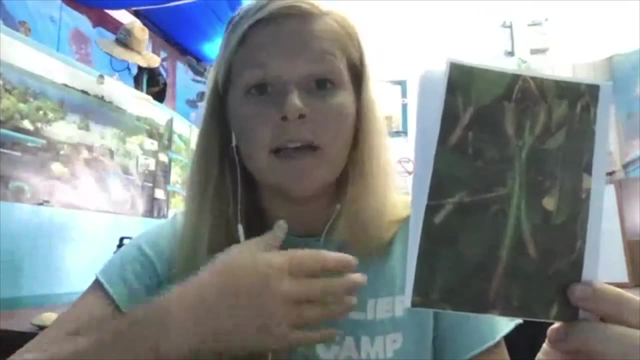 plant that has live birth And there is a special word for this. It is called viviparous. Viviparous just means that the propagule is alive, And we're going to talk about this on the worksheet, about why that's so important for mangrove. 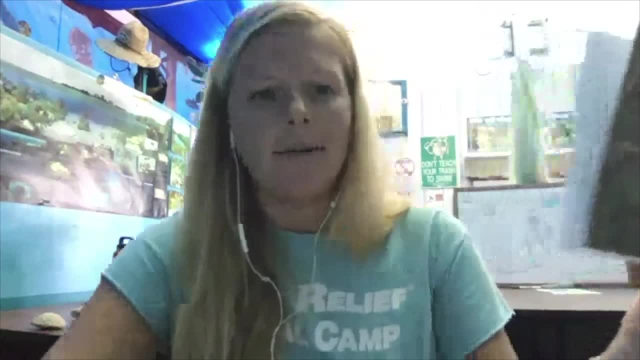 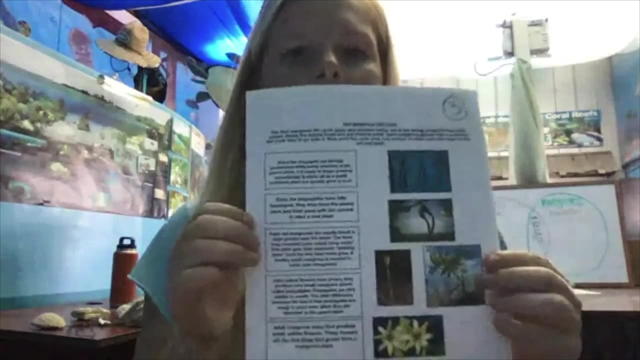 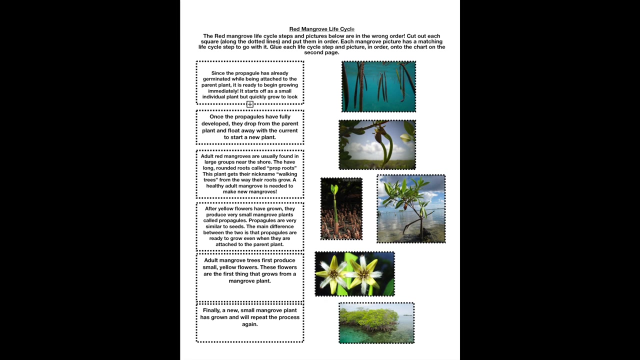 ecosystems for their propagules to already be alive. So once again, that word is viviparous. Alright, so now everyone can take out their mangrove life cycle worksheet, Which looks like this and this. So on this page, guys, there are the propagule. 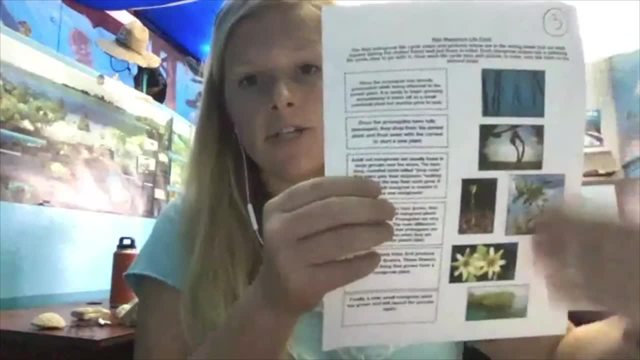 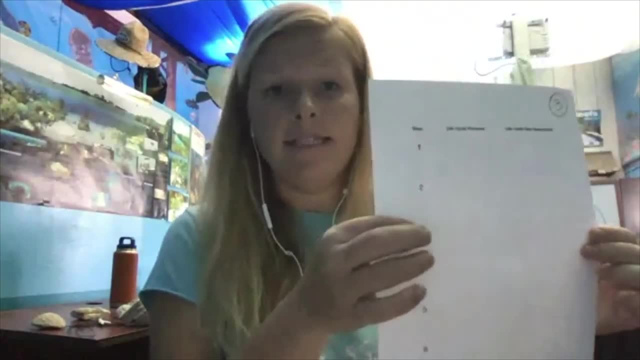 and mangrove life cycle. that's out of order, And the pictures are out of order as well. So you are going to cut out each of these squares and label them on this activity sheet right here. I'm going to help you more with the description, so 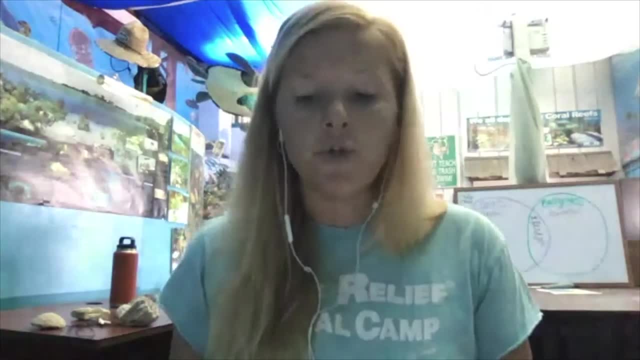 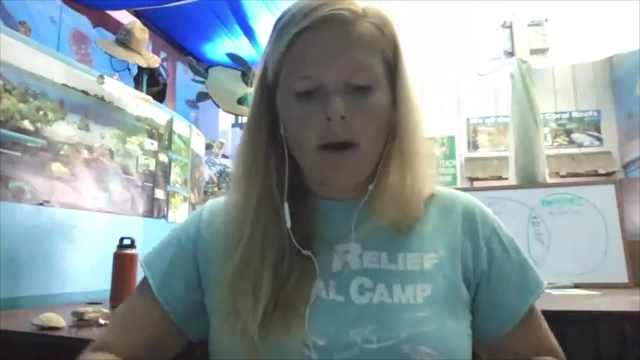 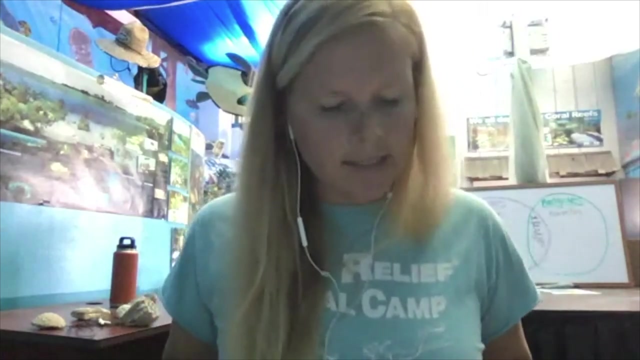 the boxes that have words in it. And then, once this is over, you guys can paste and cut out the pictures to go along with the description. So I started to cut out my description, so you guys can all start to cut out yours as well After looking at these. the first step, 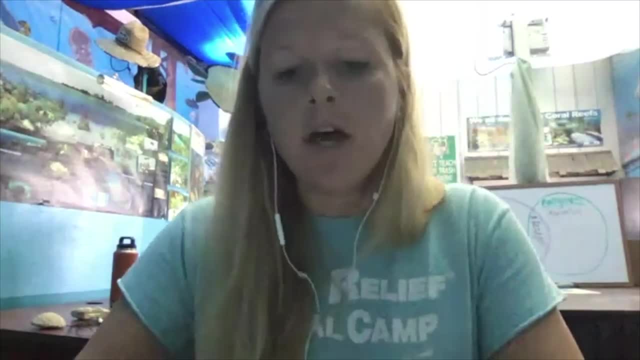 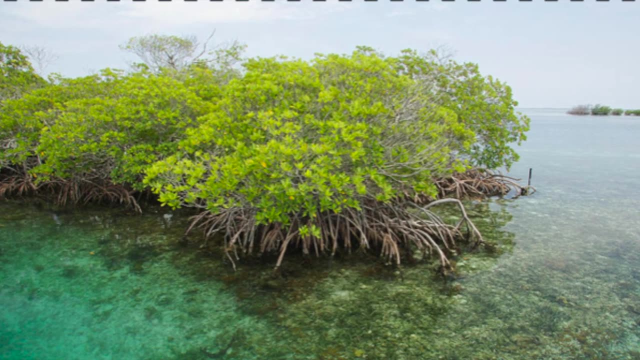 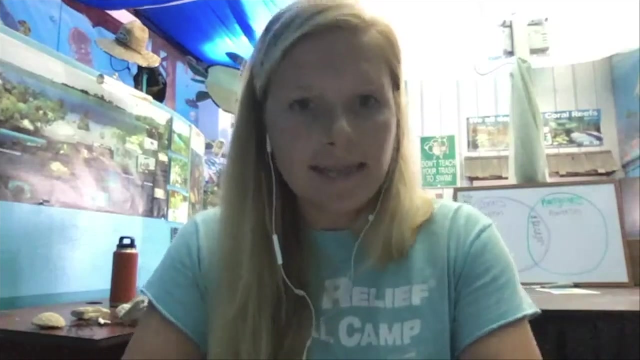 is going to be this box right here And it reads: Adult red mangroves are usually found in large groups near shore. They have long rounded roots called prop roots. The plant gets their nickname walking trees from the way their roots grow. A healthy adult mangrove is needed to make new. 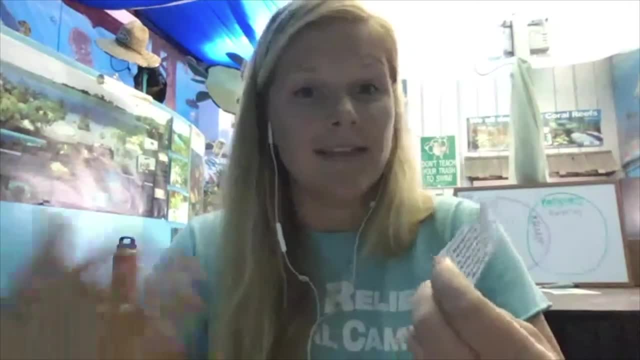 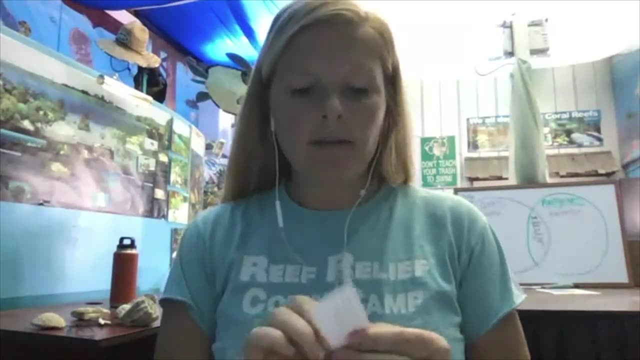 mangroves. So this is number one, because you need an adult mangrove to make these proper yields and to grow into other plants. So that's number one. So you can glue that on your step one on that second page. The second one is this one and it says: adult mangrove trees first produce small. 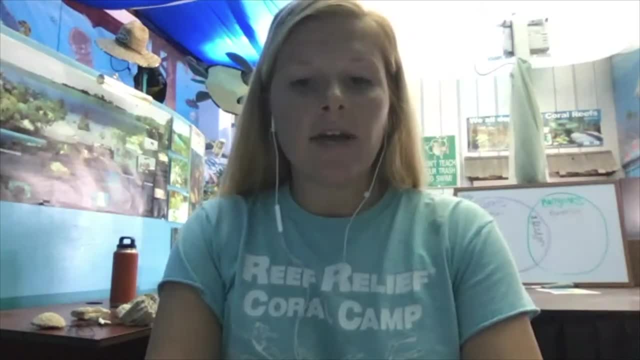 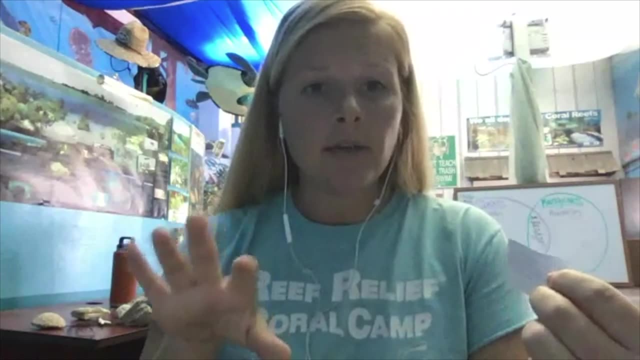 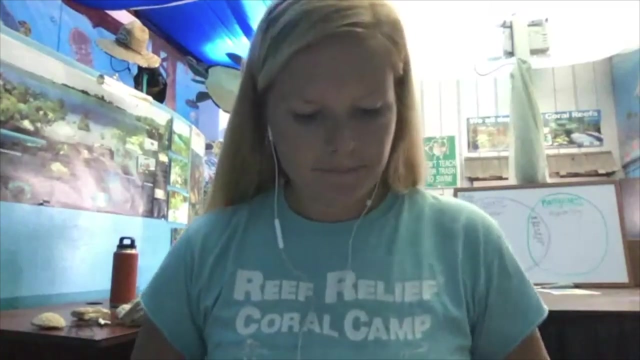 yellow flowers. These flowers are the first thing that grows from a mangrove plant, So you have an adult plant. they're gonna start to sprout or grow these little yellow flowers and that is going to be the first sign that the plant is starting a new plant- Alright, the next one. 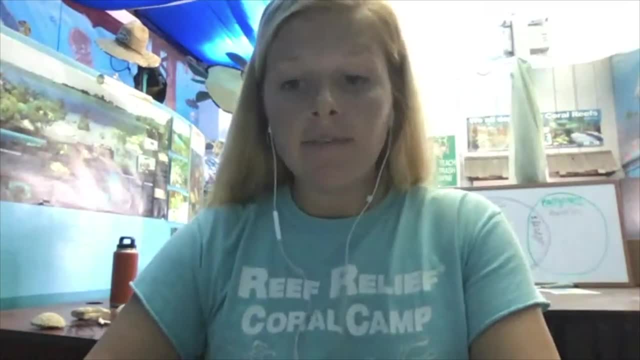 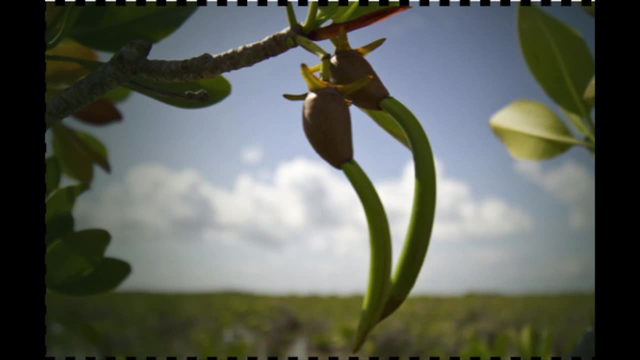 After yellow flowers have grown they produce very small mangrove plants called propagules. Propagules are very similar to seeds, but the main difference between the two is that propag realised plant is growing very small, aligning up with the contributes three plants. 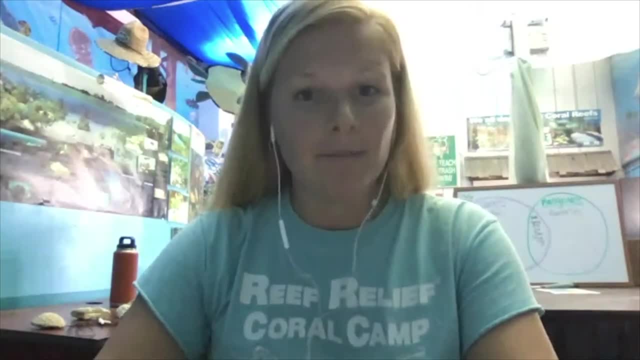 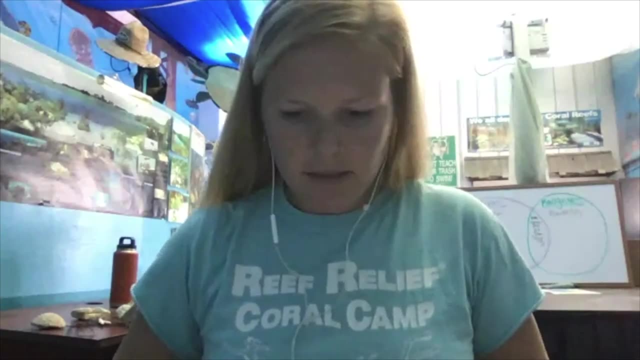 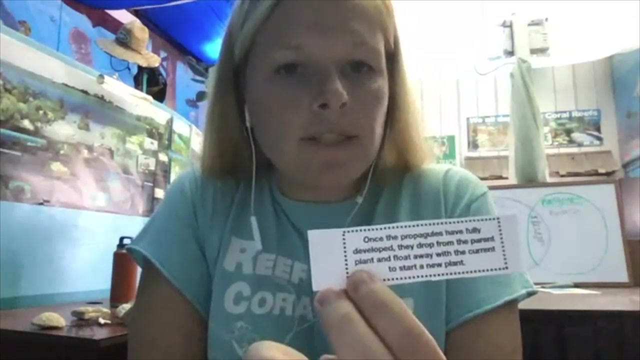 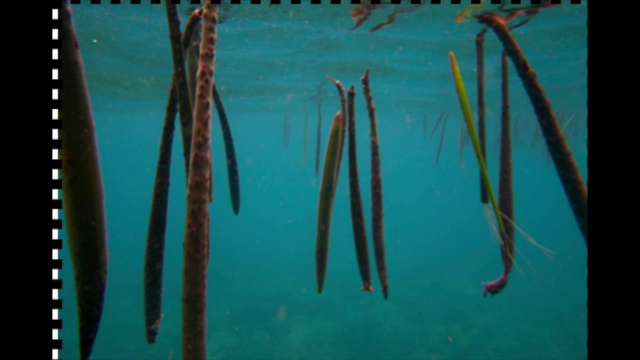 are ready to go, even when they're still attached to the parent plant. So that's the third one. The fourth one is this guy right here says: once the propagules have fully developed, they drop from the parent plant and float away with the current to start a new plant. 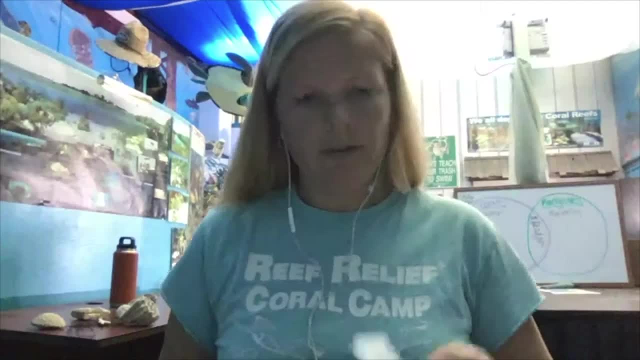 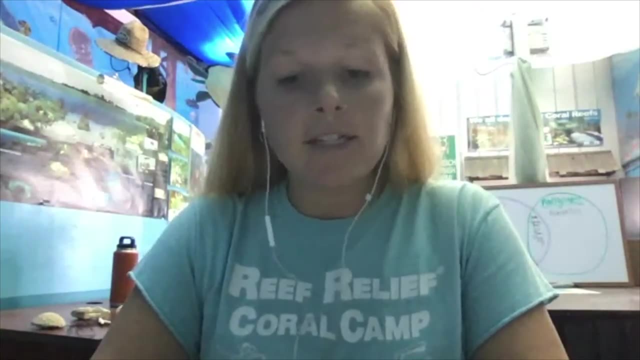 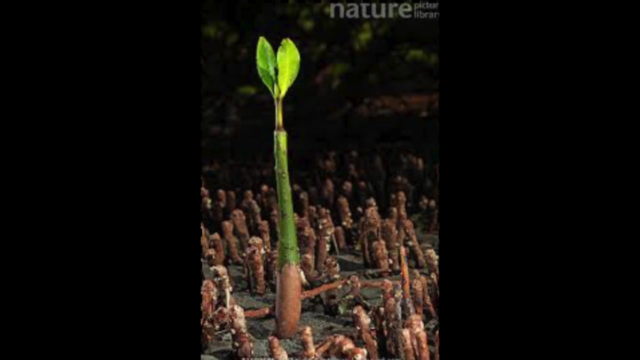 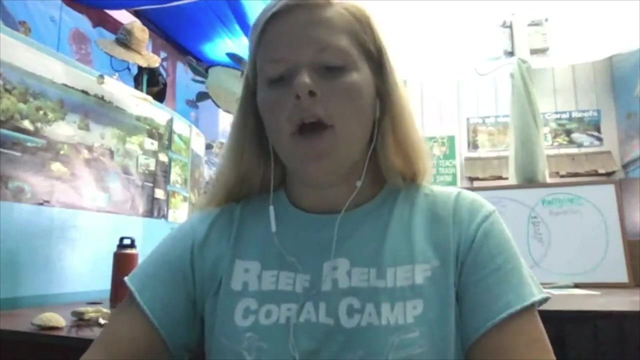 All right. and the fifth one, Since the propagule has already germinated, while being attached to the parent plant, it is ready to begin growing immediately. It starts off as a small individual plant but will quickly grow to look like its parents. All right, and finally, a new small mangrove plant has grown and will 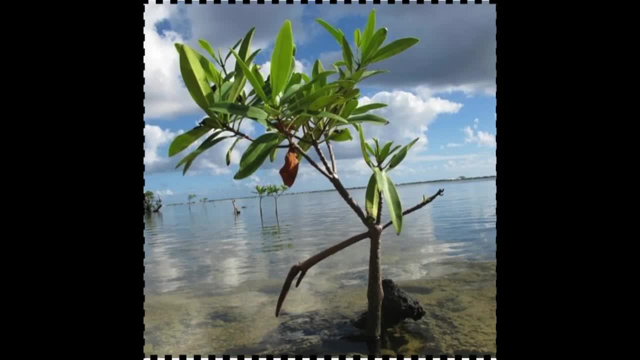 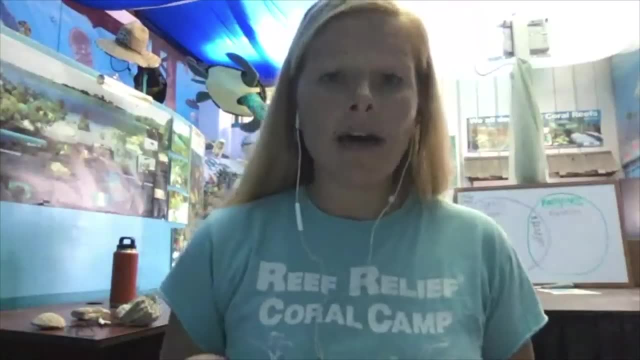 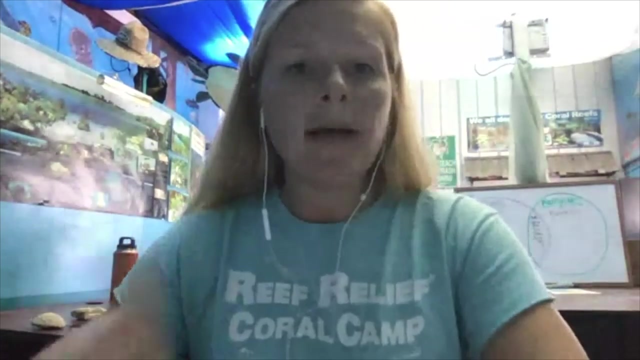 repeat the process again. so that is the final step. so after this, guys, i want you to glue them in order on the way that i just talked about it and then also find the picture that matches up with that description. so our main activity for tonight is, if you go back onto our blog,